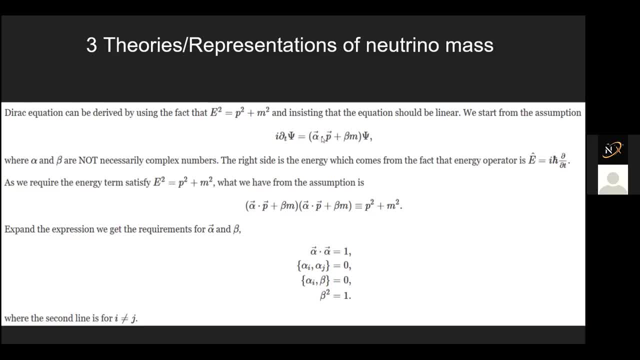 So these need not exactly be complex numbers. These can be, obviously. But yeah, in general this is the equation that you would get And if you combine that with the first equation that we took the Hamiltonian system, we would get this: 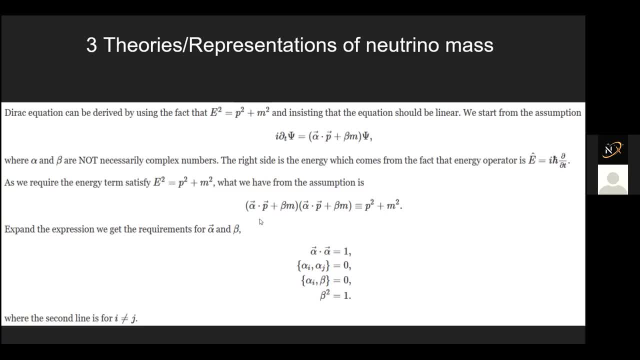 We would get this equation: Alpha plus- sorry, alpha p plus beta m, whole squared would give you this, And after you, you know, open the brackets and solve it. this is what you get Now. this alpha i and alpha j are basically for multiple values of alpha, because you would get these answers in the form of matrices. 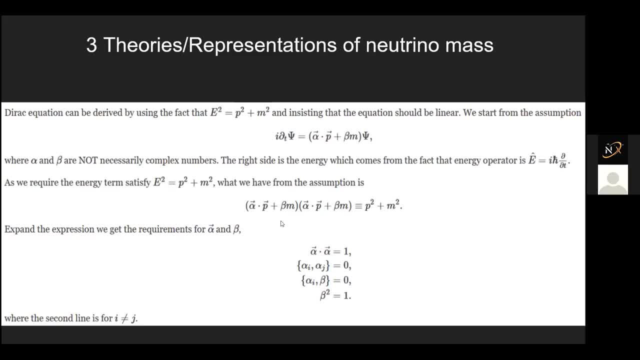 So i and j would be like sorry, you get them in the form of like a vector, So i and j would be the component number. So this is the anti-commutative property. So it's basically alpha i into alpha j plus alpha j into alpha i equals 0.. 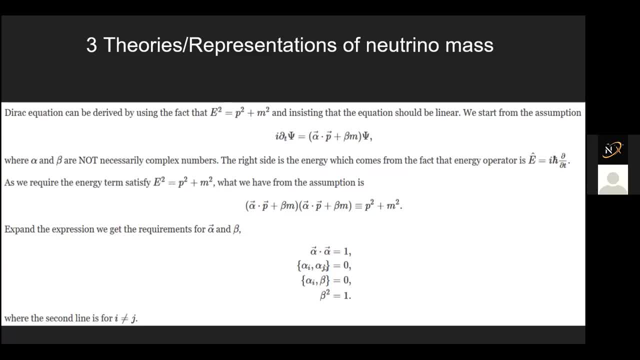 You know, for a normal commutative it would be minus, But for anti-commutative it would be plus. And the scalar product has to be 1 because of the coefficient of p squared And beta squared has to be 1 because of the coefficient of m squared. 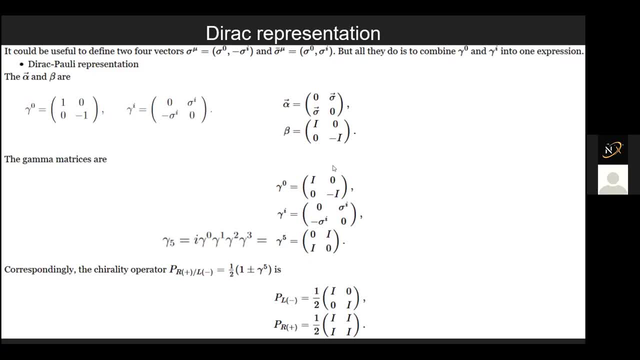 So the three representations are the Dirac representation, the Weyl representation and the Majorana representation, Named after the three scientists. So let's see what Dirac has to say about his own equation. So it would start. He would start by defining two, four vectors, sigma and sigma, covariate and contravariate ones. 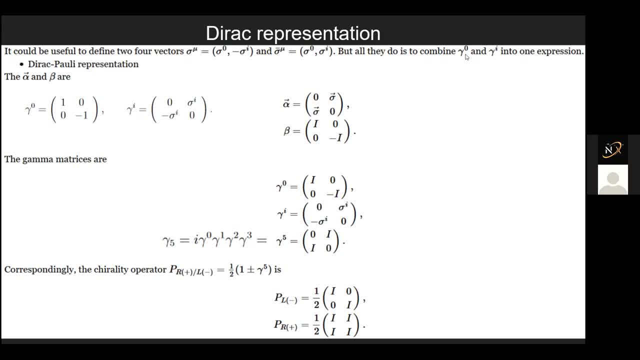 But all they do is basically combine something called gamma matrices into one expression. So the gamma matrices are matrices that are formed using the value of beta. So beta would be gamma power 0 and alpha i. you know the alpha j that you saw here. 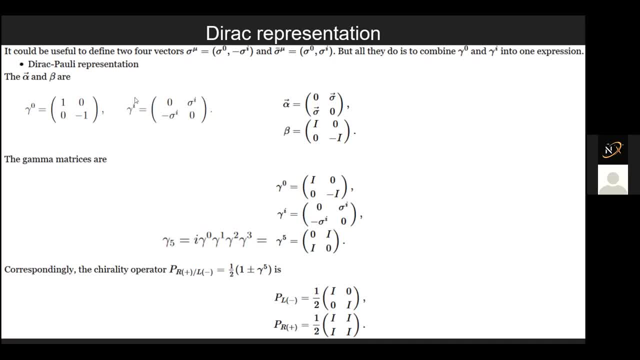 would be the gamma power i or j. So this would be like alpha i. This would be the value of alpha i. So that's the gamma matrices in general. So gamma 0 would be beta And gamma power 5.. This is not exactly power 5, even though it's written in that similar way. 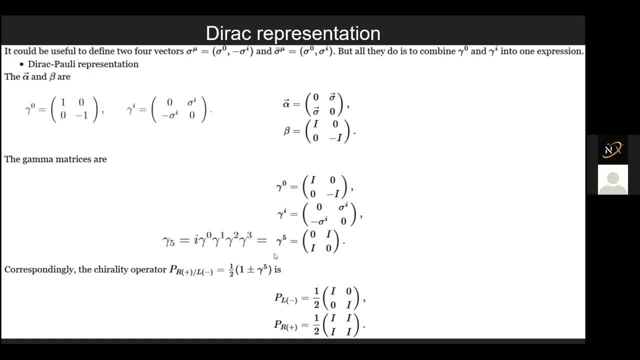 It's basically, i times, the product of the four gamma vectors. Now, why is gamma 5 important? Because that gives you the chirality operator, Meaning an operator that tells you whether a particle is left-handed or right-handed. And now we know what left-handed and right-handed are. 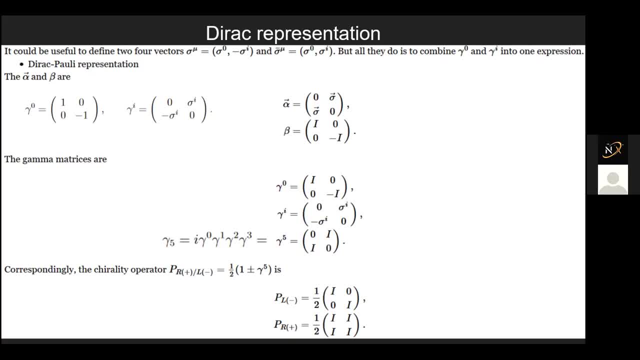 That's the chirality. Now, if a particle is moving along a direction with respect to its direction, if it's rotating clockwise it would be right-handed, And if it's rotating anticlockwise it would be left-handed. So we have an operator for that, as all of quantum mechanics does. 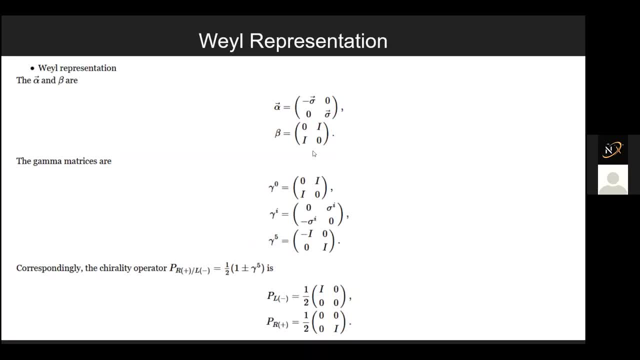 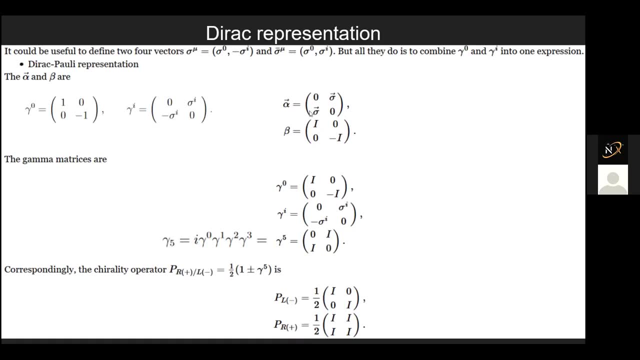 And thus gamma 5 is really important, And the second one is Weyl interpretation, And here the gamma ideas do remain the same, but there's a slight difference in the alpha, as you can see. Here is the second and the first element, but here is the first and the second. 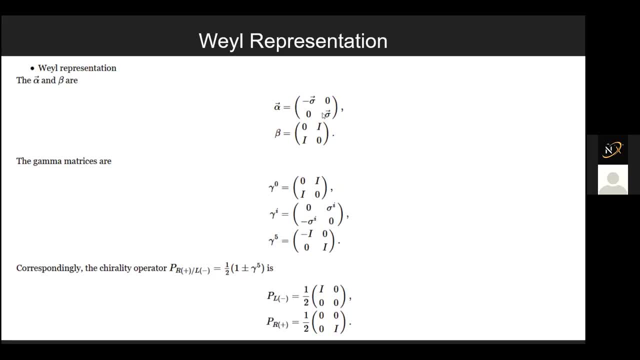 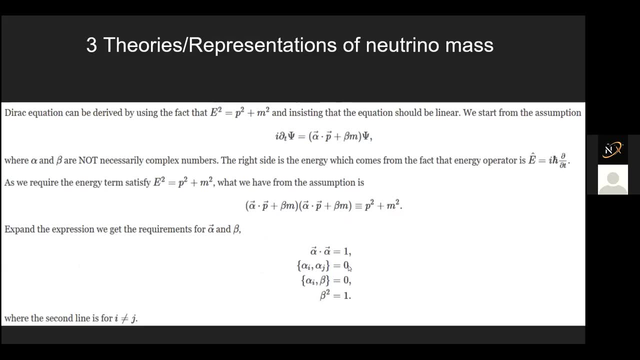 So in general, you can have gamma matrices as any random matrices, as long as they're anticommutative. They have to follow this property. Then you can follow any gamma matrices. That's why you can have multiple representations in the first place. 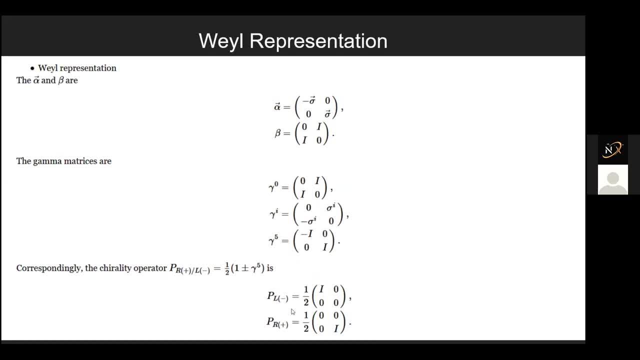 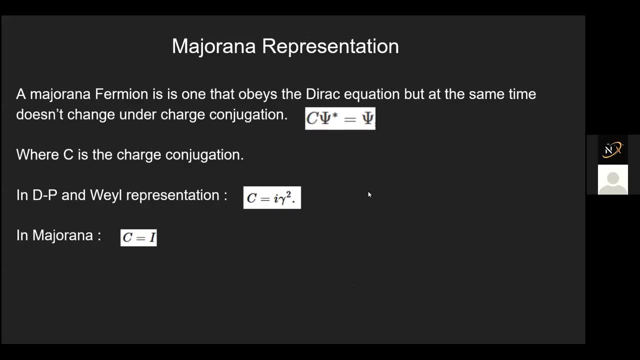 So in the second representation he does this. You get a different thing, but it symbolizes the same thing. And the third one is the Majorana representation. So what's the difference? A Majorana fermion is one that obeys the Dirac equation. 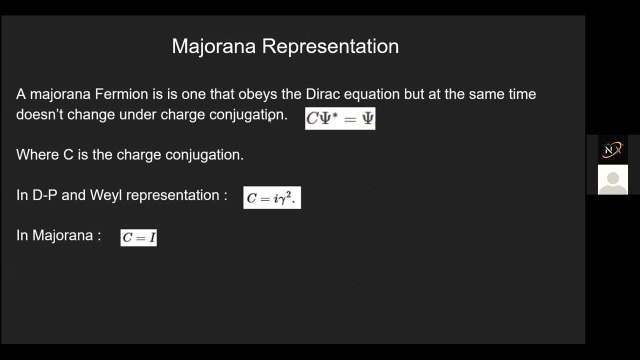 Like you know the previous two ones, But at the same time doesn't change under charge conjugation. So what's charge conjugation? That is an operator in normal Dirac poly and Weyl representation. That would be i times gamma squared. 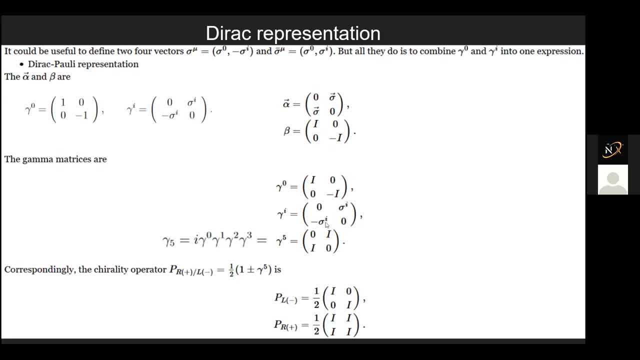 Where you know gamma squared is you know, just replace i with you know 2.. That would give you gamma squared, So i times gamma squared. it's the same for both Dirac poly as well as Weyl. 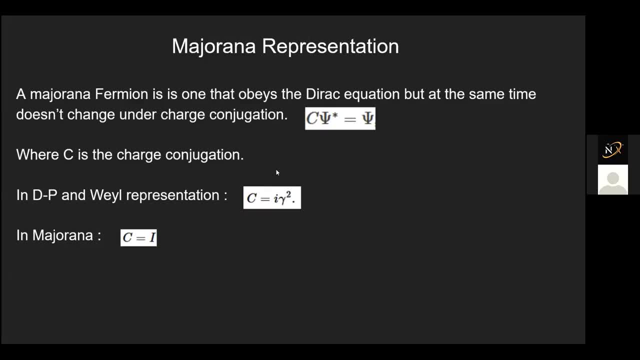 Because gamma i is the same, So that would be the charge conjugation operator. But the Majorana says that the charge conjugation operator is in fact the identity matrix, Meaning a charge conjugated particle is the same as the particle itself. 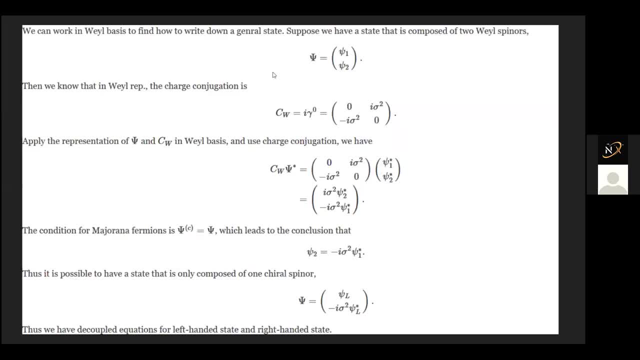 This can have some serious implications. So we can start off by proving how this is the case. You can start with Weyl. You know you can use either of them, but you're going to use Weyl here. So in Weyl representation the charge conjugation is i gamma 0, where gamma 0 is, you know, beta. 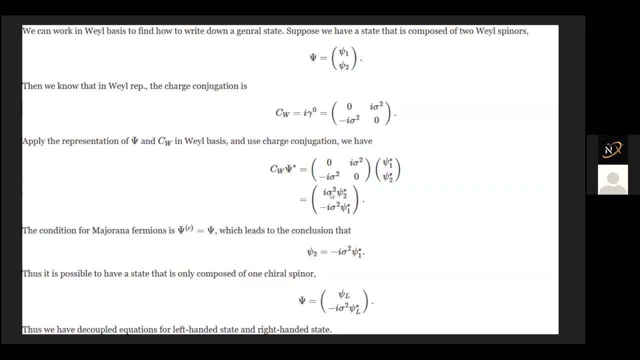 So if you apply the representation and if you use a charge conjugation, this is what you get Here. I'm saying gamma 0 because I'm using, you know, Weyl's conjugation, but I'm trying to derive the formula for Majorana. 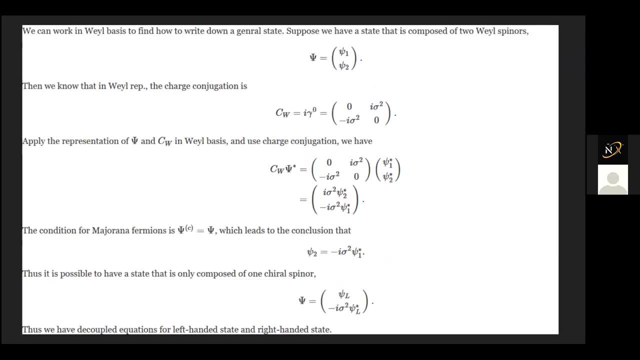 Because from you'll see why that's the reason. So if you go through the, you know, just substitute and try to open the brackets And the condition is that you know the charge operator. it gives you the same after leading to it. 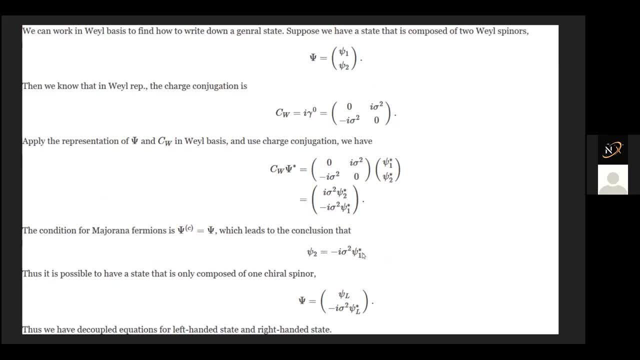 So you have: psi 2 is equal to minus i sigma squared psi star 1.. So the normal psi operator, instead of being psi L and psi R, would be psi L and psi R would be this value Minus i sigma squared psi star L. 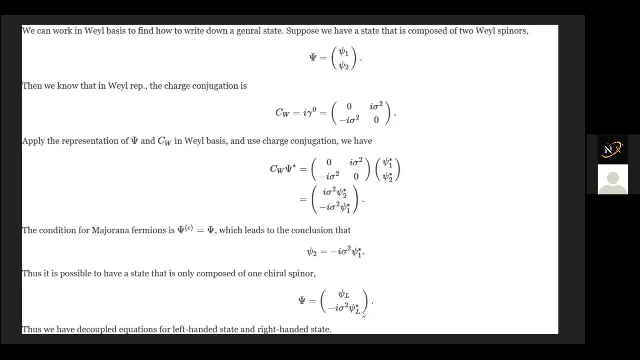 So thus we have decoupled equations for left and right-handed state Meaning we have different equations for left-handed wave functions, meaning wave functions of neutrinos which are left-handed and right-handed. So in the Dirac representation and the Weyl representation this would be the equations. 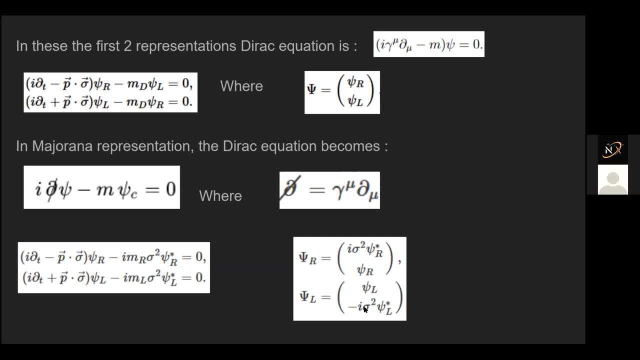 This would be the right-handed and the left-handed part, But we have seen previously how you know, right-handed can be written as minus i, sigma squared. So in the Majorana representation these would be the equations: Sigma R and sigma star R. 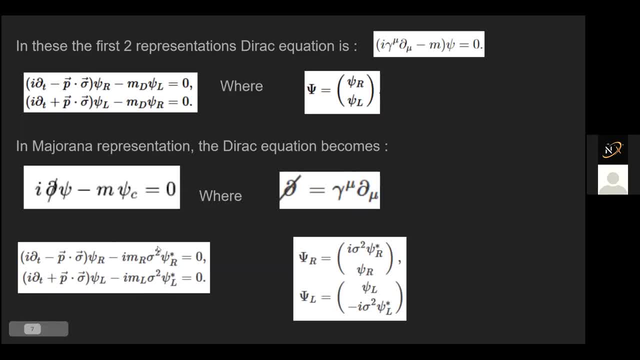 Here it would be sigma R minus sigma L, But here there's an i sigma squared in this representation. These are just fancy symbols that I won't really go over, because if you see a general Dirac equation, this is what the equation would be. 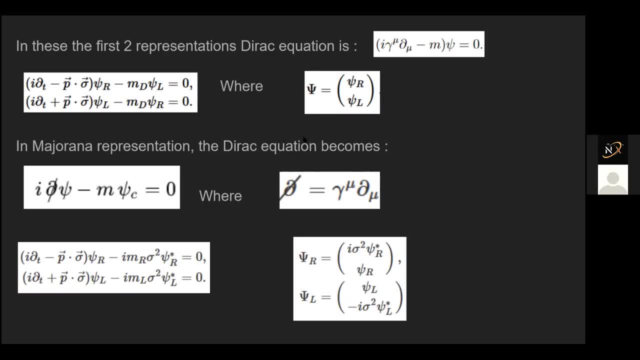 Gamma power. mu is the, you know, the gamma matrix, Gamma matrix with the mu index, And that you represent in the Majorana form. in this way, It's basically mu times dou mu itself, But here it's just that you express it in the form of this conjugate instead of the normal wave function. 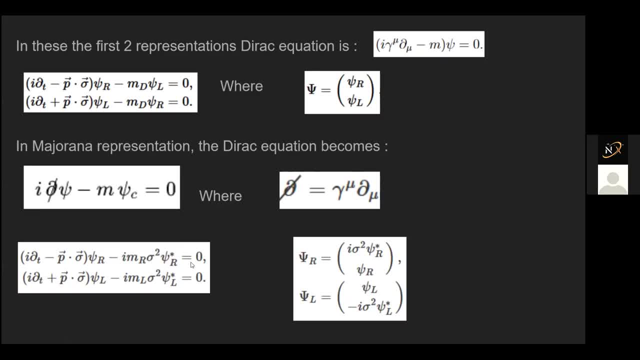 And that conjugate would be minus i sigma squared. you know that conjugate. So the idea is, you try to express an equation in the same handedness, in the hopes of achieving something, And he does achieve something, And that is the. that's what you're going to look at. 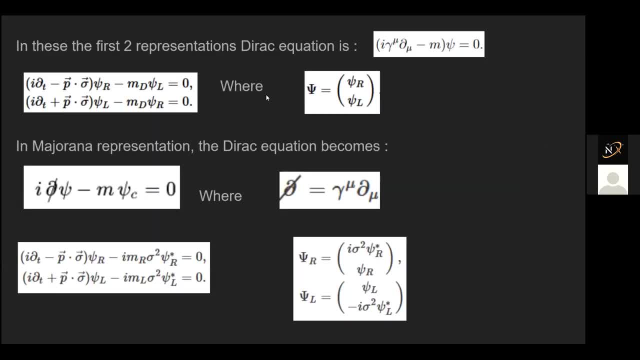 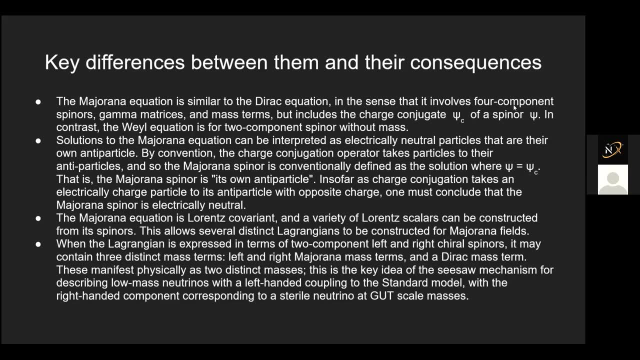 So what's the key difference between them? I mean, we did see the key difference. You're trying to express it in a different way, But what does that actually imply? So a Majorana equation is similar to the Dirac equation in the sense that it involves four components: spinors, gamma matrices and mass terms. 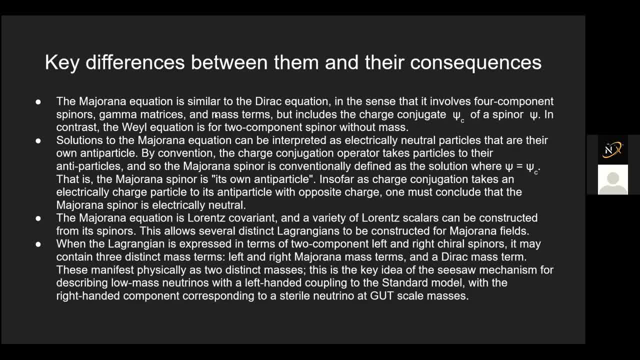 So here you assume xi to be a spinner. So basically a spinner is. you could think of it as something similar to like a vector or a tensor, But it is a component that is more related to the negative rotation of a thing as opposed to its, you know, magnitude. 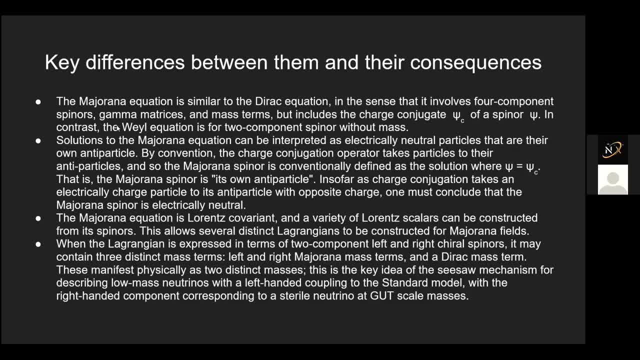 For now. you could think of it as just a normal rotation. You could think of it as just a normal wave function. It doesn't really change the meaning much So gamma, matrices and mass terms. But it includes the charge component psi c of a spinner psi. 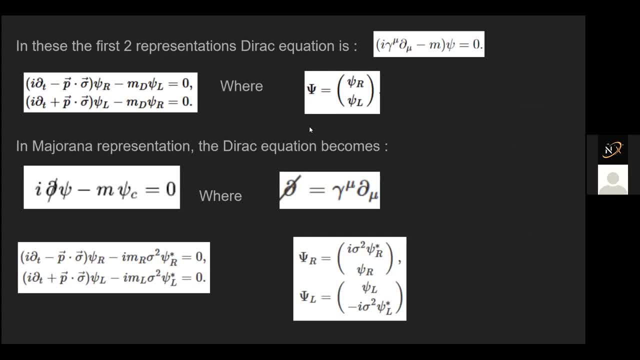 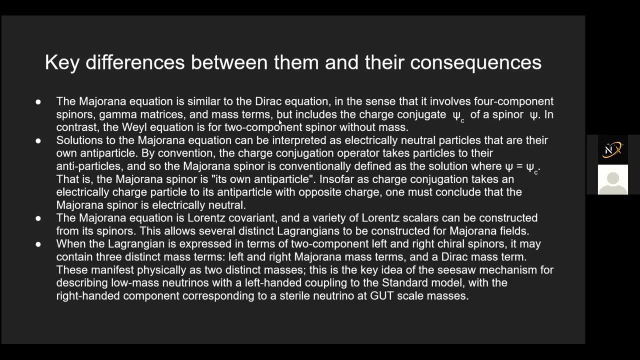 So psi c wasn't there in the Dirac equation But it's there in the Majorana equation. So that's one of the key changes. And the Weyl equation is for two component spinors without mass. I haven't included that. 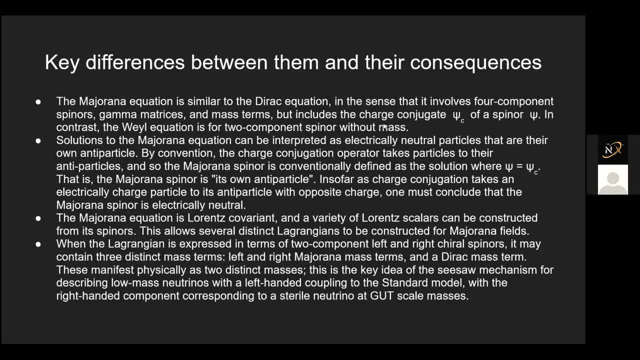 I've just done the Dirac equation, because the whole point is mass And there's no point talking about the equation without mass. The solution to the Majorana equation can be interpreted as electrically neutral, As electrically neutral particles, That's their own antiparticle. 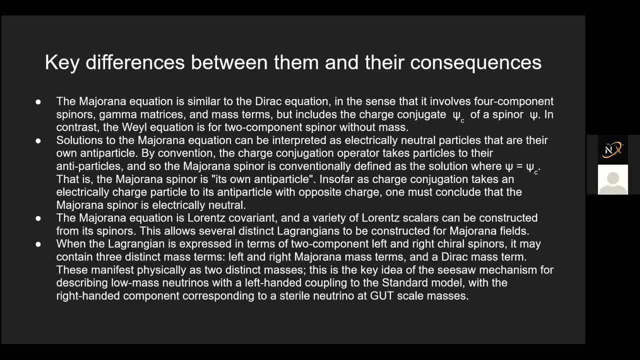 So a charge conjugation is not necessarily just switching an electric charge. There are all sorts of charges. There are color charges, There are weak charges, There are weak hypercharges, And all of them. So if you invert all of them, that would be, you know, calling it a charge conjugation. 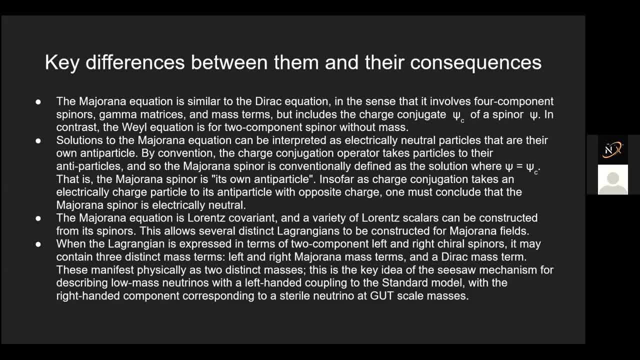 So if you know, you say a particle's charge, conjugation is an identity matrix, it means the charge you know. if you invert all of those charges then the particle remains the same. And what happens if you invert all known charges? 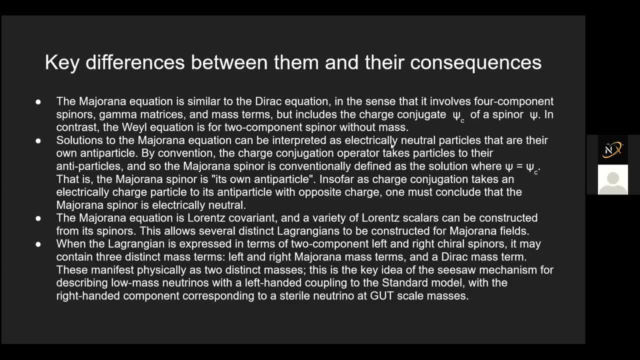 You're going to get an antiparticle of the said particle. So what Majorana really says is that neutrinos are their own antiparticle. You know, like it's called a Majoron, Like a fermion, a Majorana fermion. 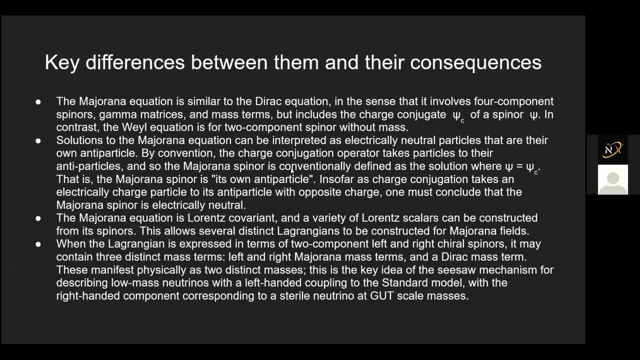 So it's called a Majoron. So that has some very deep implications. Majorana spinor is its own antiparticle. Insofar as charge conjugation takes an electrically charged particle to its antiparticle with opposite charge, one must conclude that the Majorana spin is electrically neutral. 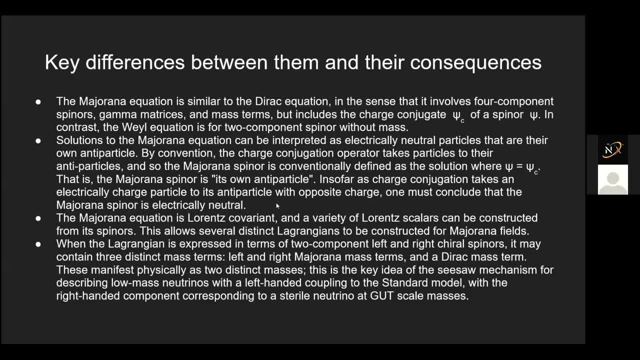 So if it's its own, you know antiparticle. so you can't have a plus antiparticle having a plus charge. It has to be minus charge. So you know, if X is equal to minus X, this is possible only if X is equal to zero. 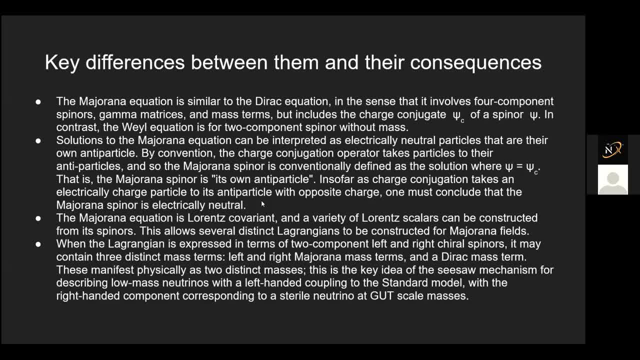 So we know that a Majoron has to be neutral. So this system does not apply to any of the charged leptons. Like any of the charged fermions- Fermions for that matter- It has to be a neutral fermion And that's called a Majoron. 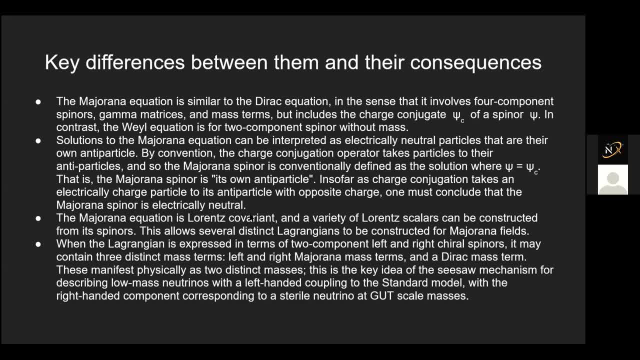 A Majorana equation is Lorentz covariant. This is not Lorentz invariant. It means it does change under Lorentz transformation And you do get you know corresponding matrix And a variety of Lorentz scalars can be constructed from them. 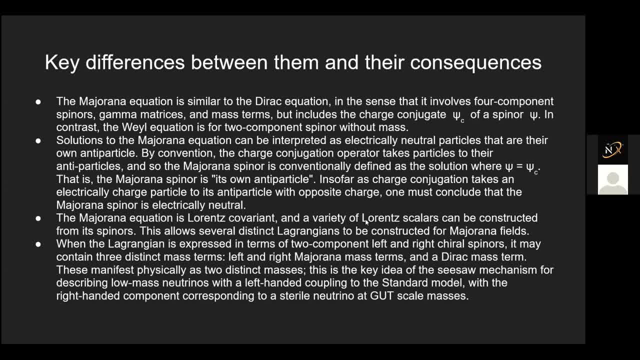 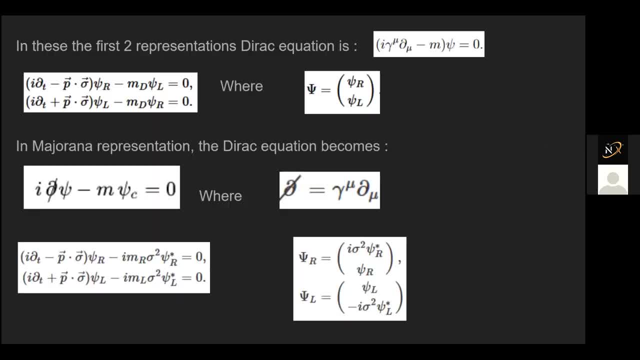 This allows for several distinct Lagrangians. I'm not going to go into detail of this, But because we have seen that you know left and right handedness there is a difference, You know it's not the same Here, left and right would be both incorporated in one equation. 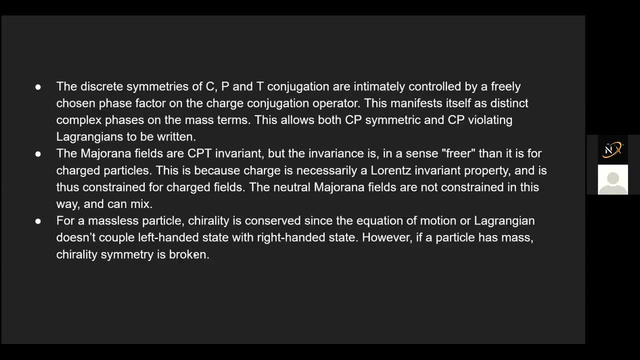 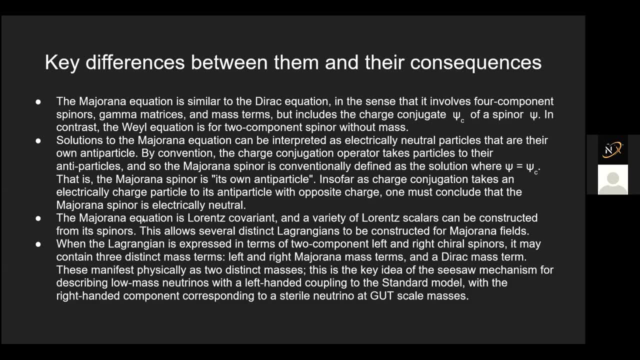 But here there are two different equations. So they have their own, you know, set of laws, And so there's their own fields. So that is what the sentence is trying to say. Then, when the Lagrangian is expressed in terms of two component, left and right, chiral spinors. 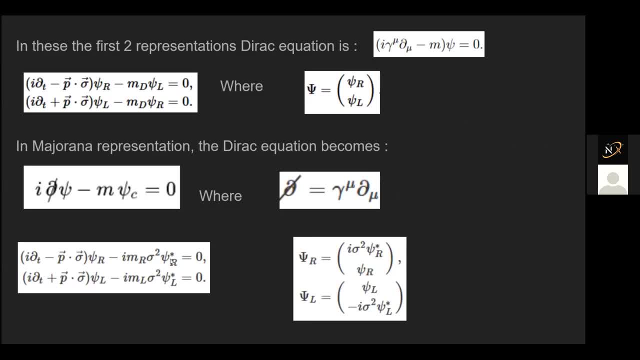 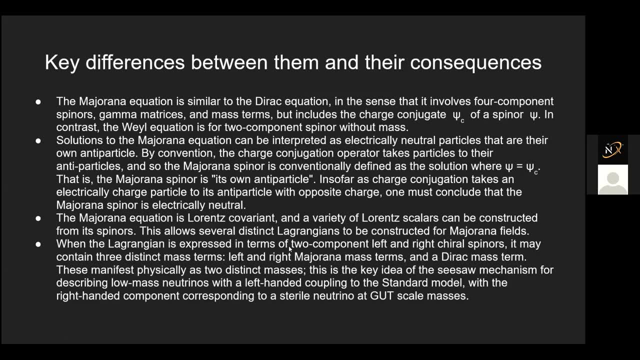 it may contain three distinct mass terms Here. three distinct mass terms- Okay, not there, I will show later. The one would be the normal Dirac mass term. The Dirac mass term is basically what the standard model predicts. It would be the mass of, say, a fermion. 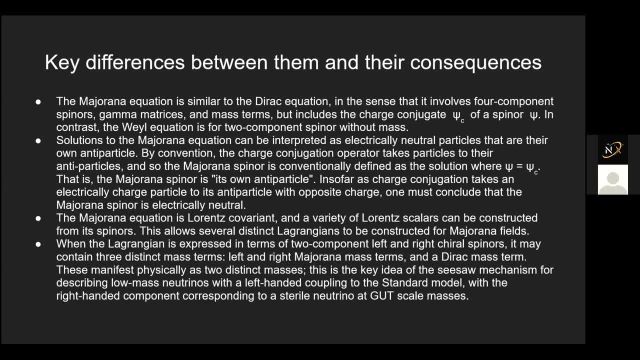 Sorry, a lepton, a charged lepton, Like an electron neutrino mass. The Dirac mass would be similar to that of an electron itself. That's the major, you know, problem with standard model. You can't even tell why the neutrinos are so low mass. 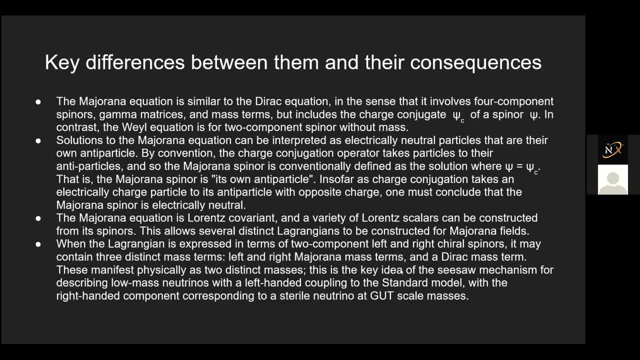 These manifest physically as two distinct masses. This is the key for the idea of seesaw mechanism. Now I'm going to go in depth about seesaw mechanism in a bit And I'm going to only type one. We're describing low mass neutrinos with a left-handed coupling to the standard model. 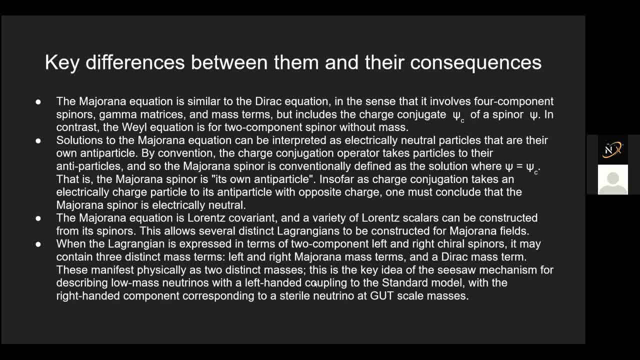 What do you mean by coupling to the standard model? Coupling would be any sort of interaction, right, And the standard model has the four fundamental forces that describe the. you know the interactions. So if you couple left-handed coupling, this means that only left-handed majorons, meaning neutrinos, interact within the standard model. 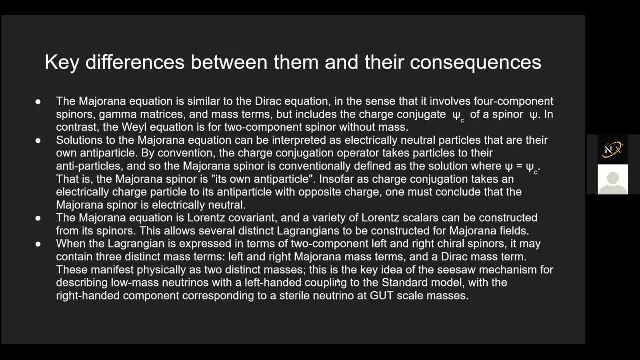 So only left-handed neutrinos, you know. you know that. you know only left-handed neutrinos react to the standard model And right-handed neutrinos react to the weak force. So that's what that sentence was, With the right-handed component corresponding to a sterile neutrino at GUT. 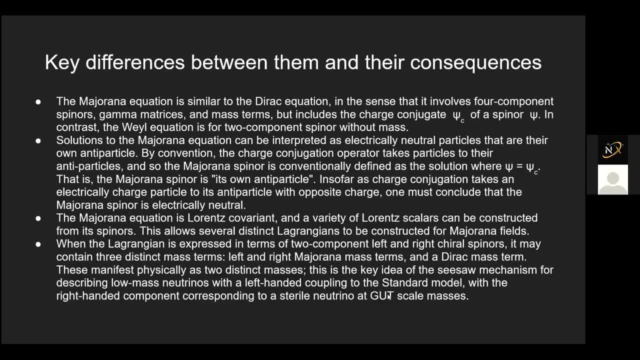 This is grand unified theory. You know, those scales were early universe with very high temperature, with like Planck energy, And the mass of the right-handed neutrino is supposed to be this, you know, as predicted by seesaw mechanism, which I will talk about. 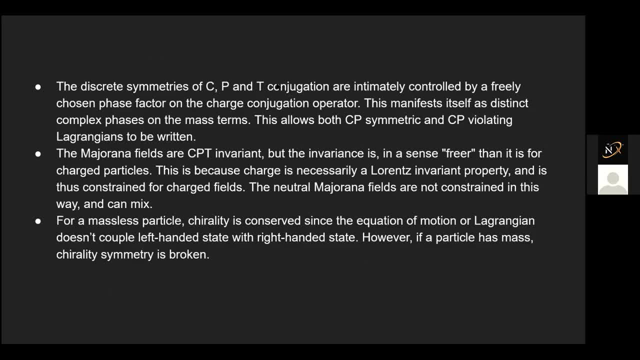 And another is the discrete symmetries of charge parity and time conjugation. The charge is, as I said, the charge electric, weak, hypercharge, whatever. So the charge electric would be invariance under shifting of the coordinate system and changing it into opposite. 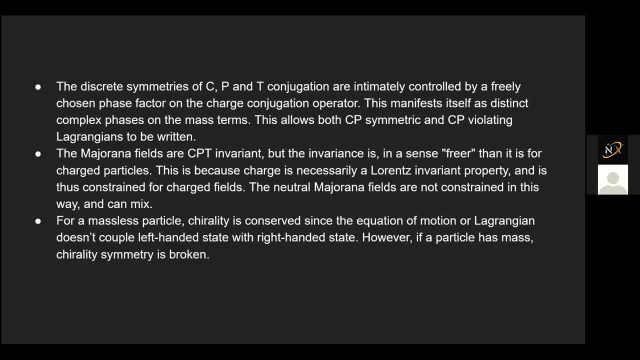 So this would be like a left-handed being a right-handed in our case, But it could in general. it's x changing to minus x, So it's like a mirror image. And time conjugation are. you know, time forward and backwards are intimately controlled by a freely chosen phase factor. 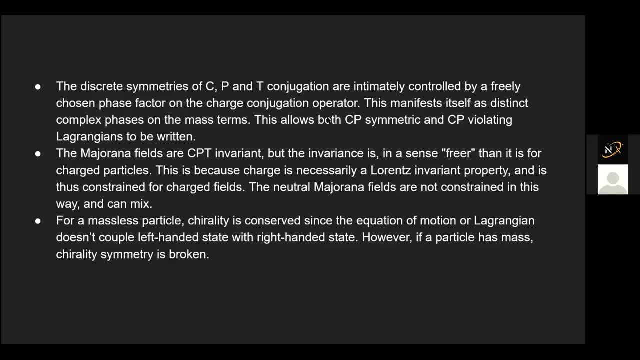 This leads to CP symmetric and CP violating Lagrangian. So basically, there's a there's, no, there's no, there's going to be a factor In the coming equations. I just want to build up the theory for that part. 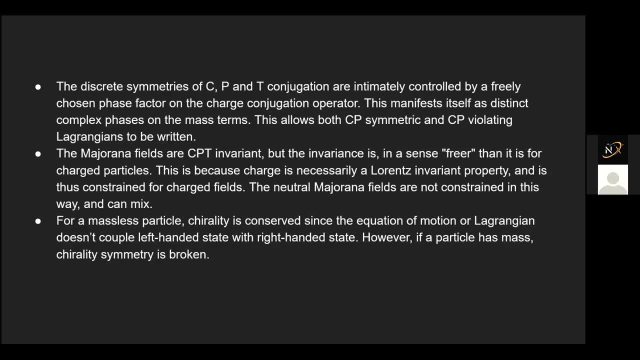 So that factor is not exactly fixed because we haven't observed, you know, the key component needed to prove major or anything, And that is the beta, the neutrino-less double beta decays. Those haven't been absorbed. So as of now they are freely chosen phase factors, meaning there's a phase out and they're not yet, you know, have a fixed thing. 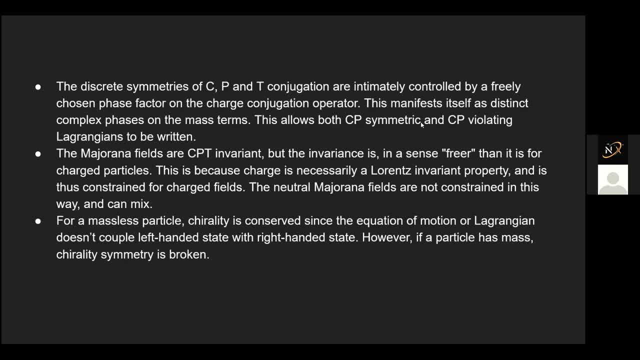 This allows for CP symmetric and CP violating Lagrangians. CP symmetric because if you have the phase factor, as say pi by 2, then all the signs would be all the sign values would be 1.. But if you have it as cost, then all of them would be 0.. 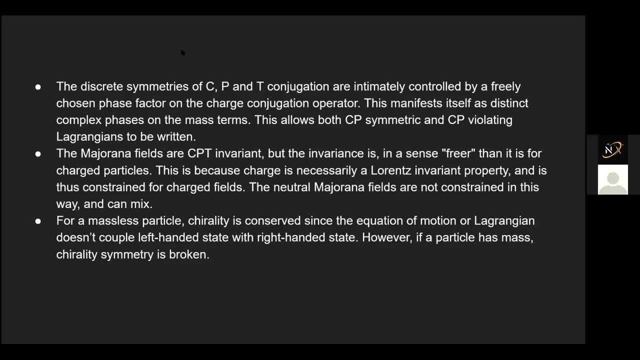 So this allows for CP symmetric as well as CP violating Lagrangians. CP would be charge and parity. If you switch both of them, they are supposed to be invariant. That's what CP conversation says. The major nanofields are CPT invariant. 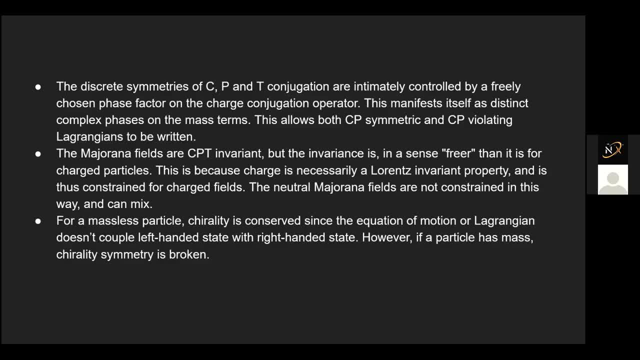 But the invariance is in a sense freer than it is for charge particles because again, charge is 0. So you just have to worry about parity all the time. The neutral major nanofields are not constrained. They are constrained in this way and can mix. This also explains Newton oscillations and mixing through this. And as a bonus, it's also Lorentz invariant. So the major theory of masses in the seesaw mechanism is a very, very powerful and likely likelihood of it existing. 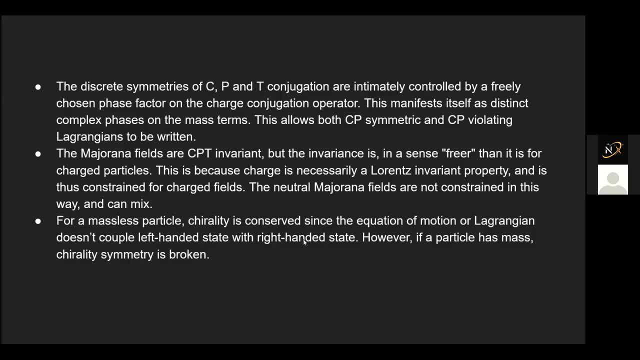 It's just that we haven't seen it yet. So for a massless particle, it currently is conserved. You know, it's like a photon, It's just spinning one way. There's nothing to it. However, if it is, 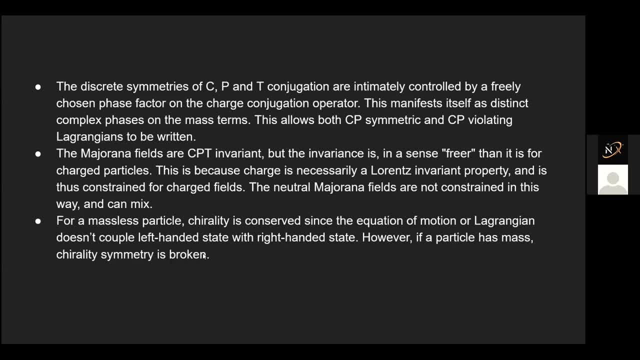 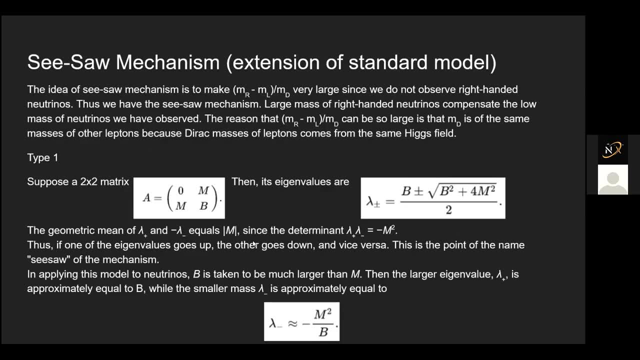 if it does have a mass, then chirality symmetry is broken because of the mass terms that I'm going to talk to you about. Okay, so the seesaw mechanism: It's an extension of the standard model, because this is not within the standard model yet. 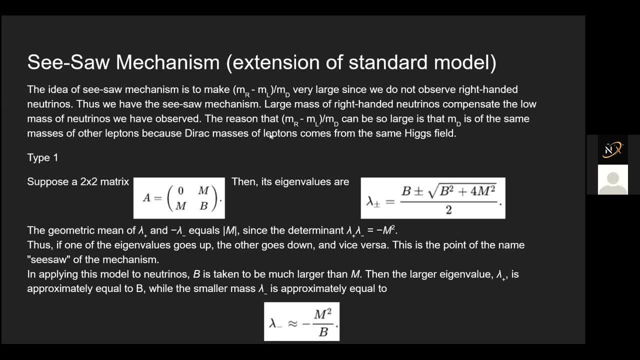 So the idea of the seesaw mechanism is basically you are going to have two different masses for a right-handed and a left-handed neutrino And you're going to have a Dirac mass, meaning the proposed mass, which is the same of the corresponding charged lepton. 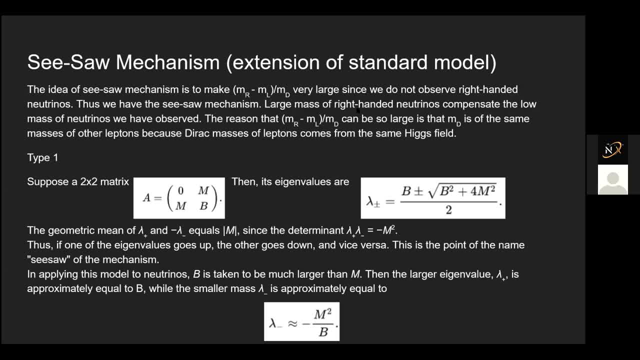 So if you try to have MR minus ML very large, because you know we don't observe right-handed neutrinos And we can just you know, we might say this is due to its inertness, And that inertness can be explained by high mass. 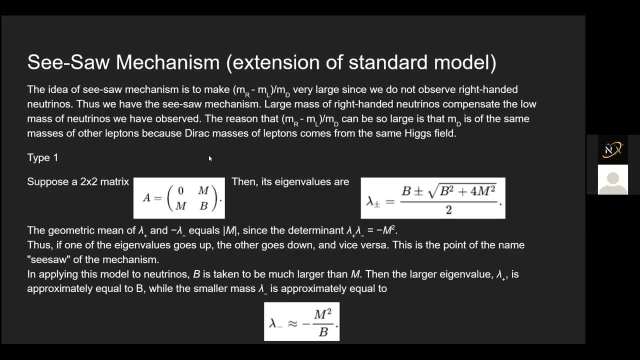 So thus we have a seesaw mechanism, So type 1.. This is what we're mostly going to be dealing with, And the reason we try to do this is because the Dirac mass comes from the Higgs field. The MD part, proposed part of the charged lepton, comes from the Higgs field. 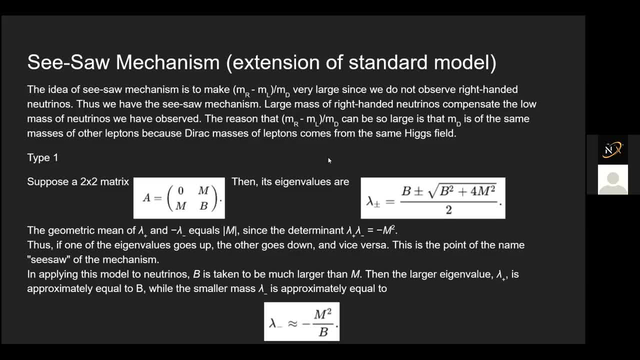 Whereas MR or ML does not. Okay, So we are free to choose what we want, And the type 1 theory that we have chosen for convenience is this. So before that, I want to talk a little bit about the diagonalization of matrices and how to get the eigenvalue of a matrix. 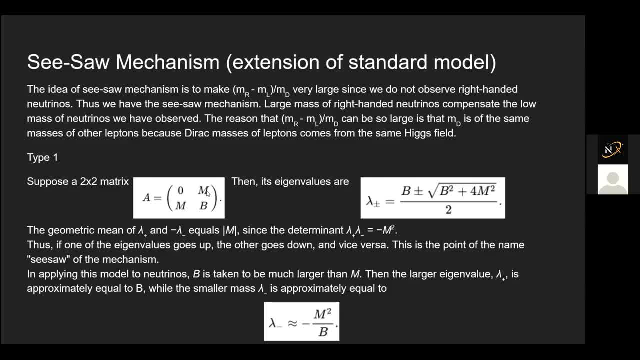 So if you have a 2x2 matrix, you can express this as a diagonal matrix of the form you know: lambda 1 and lambda 2, or lambda minus and lambda L, Lambda minus and lambda plus. So basically you're trying to express the entire A matrix in just diagonal elements. 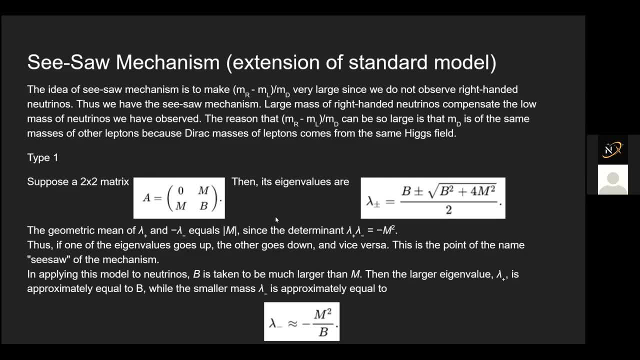 And these two diagonal elements are called the eigenvalues. So basically, these are the possible solutions of a matrix, so to speak. So it's eigenvalues For a 2x2 matrix. this is given as the general formula, which is of this form. 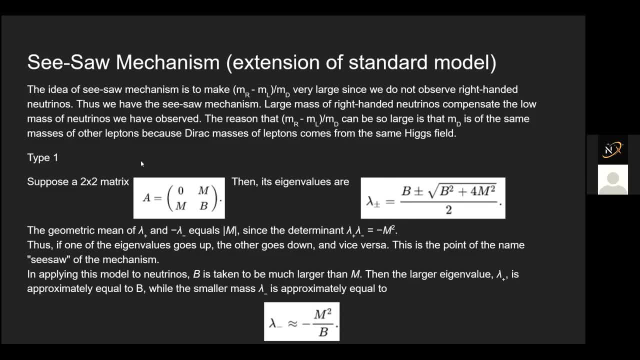 B plus minus root of B squared plus 4M, squared by 2, because you try to get the determinant And that determinant is 0 in this case. So it would be pretty easy to solve this: 0 in this case, as in after diagonalizing it would be 0.. 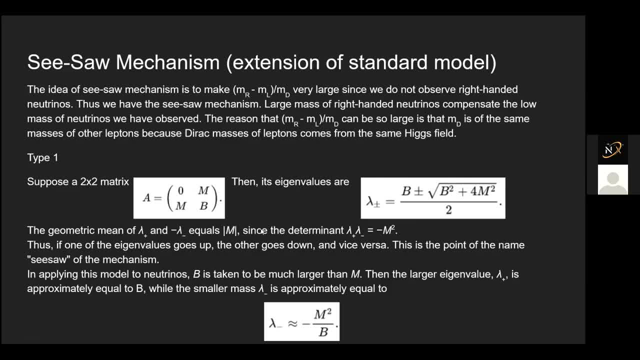 So the geometric mean of lambda plus and minus, lambda minus equals mod M, Because the determinant is 0.. Because the determinant is minus M squared, Because, as I said, you're going to express it only as lambda minus and lambda plus. 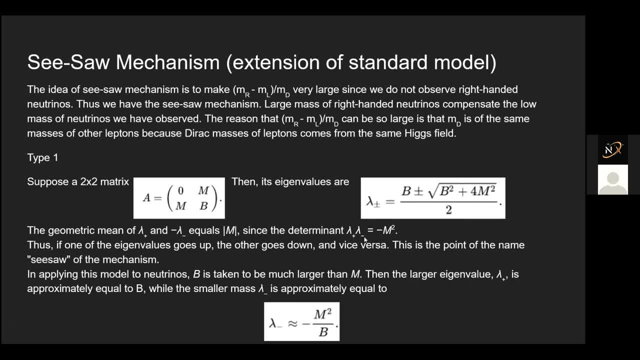 So the determinant is just going to be M squared. Thus, if one of the eigenvalues goes up, meaning if lambda plus is very high, then automatically lambda minus goes low. Or if lambda minus is high, then lambda plus goes low- 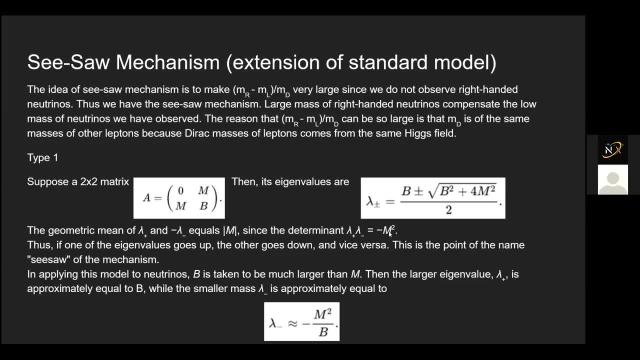 Because the product of there should be a constant. Here, M is the. when we go later it's going to be the Dirac mass. So this is called the CISO mechanism. This is the point. So the M acts as a- you know, a pivot. 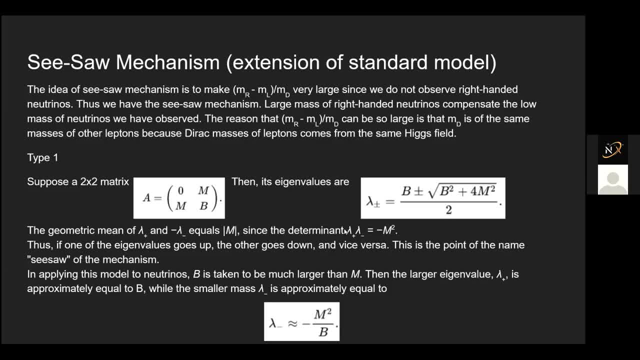 And the masses of lambda plus and minus can keep Going up and down, But if one goes up, the other has to go down. That's the reason it's called the NaM CISO mechanism, So you can apply this model to neutrinos. 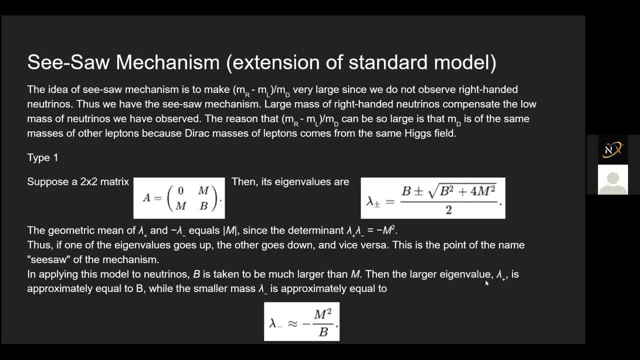 If you take B to be very, very large compared to M, then the large eigenvalue lambda plus is almost approximately equal to B, Because you see, lambda plus, if you take plus, it's just B, Because this term vanishes, because it's very, you know, small compared to this. 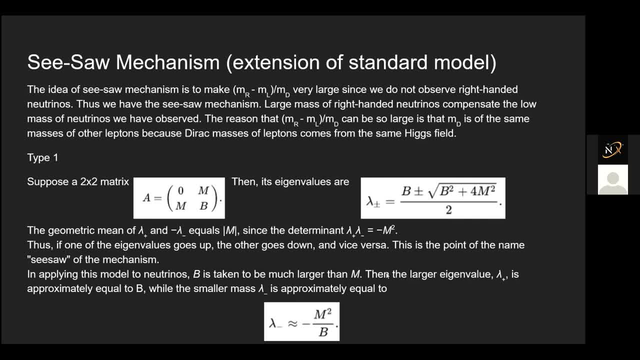 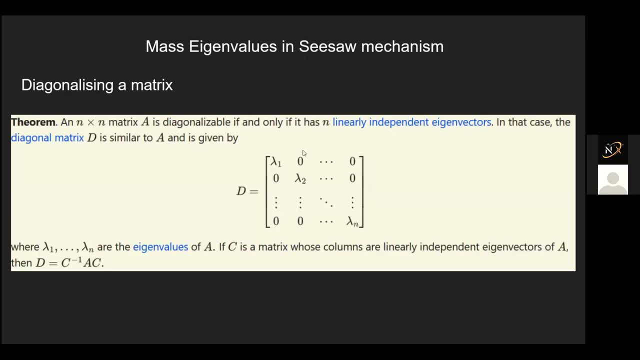 So you're going to have B plus B by 2, which is just B, And the minus part is going to be approximately M squared by B. Okay, So diagonalizing a matrix. So this is I'm just what I said previously, just to visualize it. 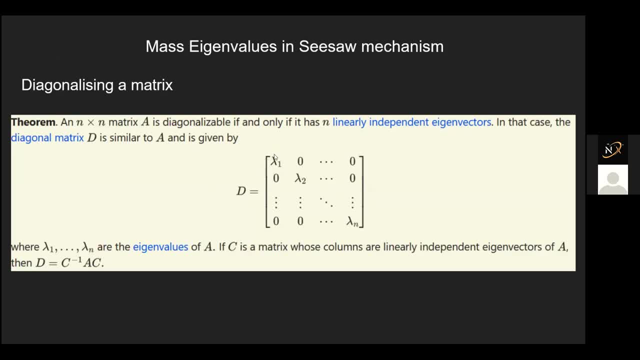 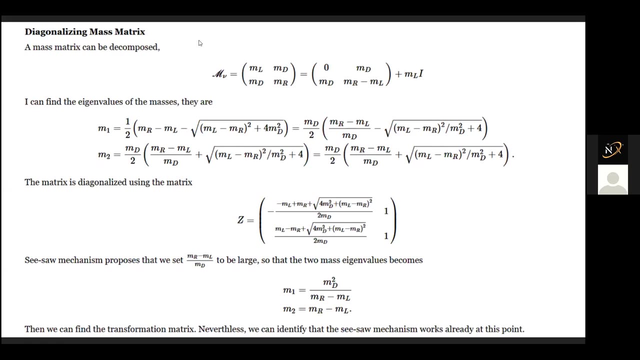 This is how you're going to get as a diagonalized matrix. Lambda 1 and lambda 2 are here, lambda minus and lambda plus, So these eigenvalues would be the possible solutions of this matrix, so to speak. Okay, So now how do you diagonalize a mass matrix? 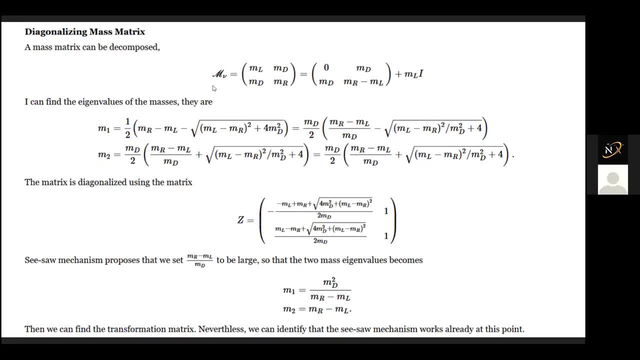 Now we get to the real part. So you can assume a mass matrix is called the Majorana mass matrix. Okay, So you can assume a mass matrix as comparing as ML, MR in the diagonal elements and MD being the Higgs masses. 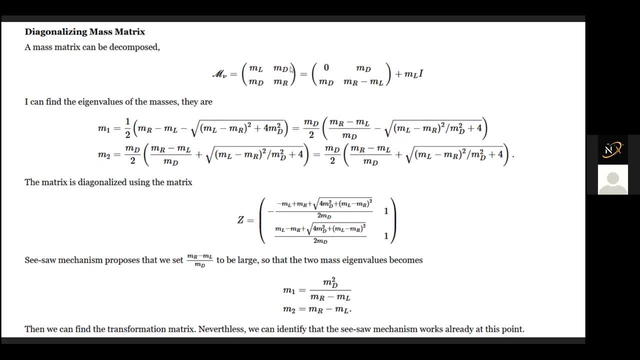 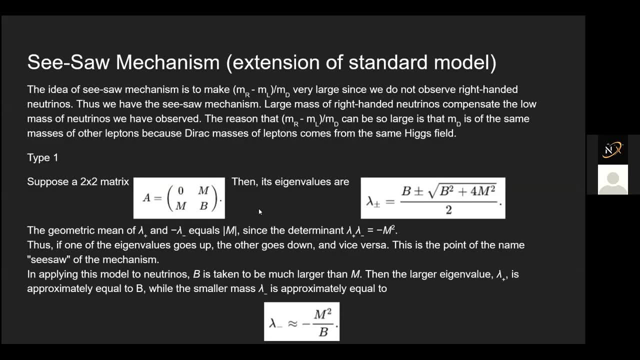 You can subtract it with you, can you know? subtract it with plus MLI and minus MLI, So you get this out. The whole idea is because you want to get this term as 0, to get it in the form of what I had expressed here. 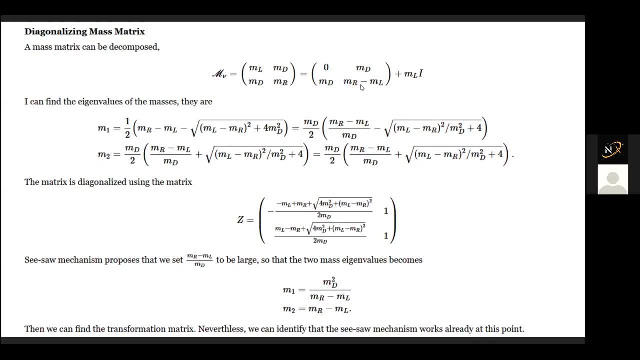 So you can use the formula directly. So if you get that 0, then MR minus ML would be your B from the previous equation, and MD is just your M. Okay, So, because you're simplifying all of that, the eigenvalues, this would be lambda minus that you saw there and this would be lambda plus. 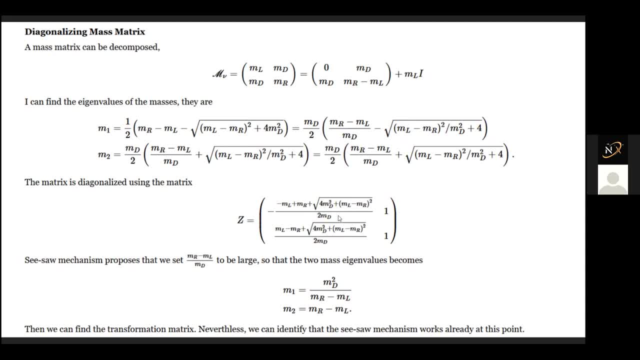 So basically, you just open it, you solve it. There's really not much complicated math here, It's just adding, subtracting and dividing. That's all this is. So see, some mechanism. This is what you get essentially. 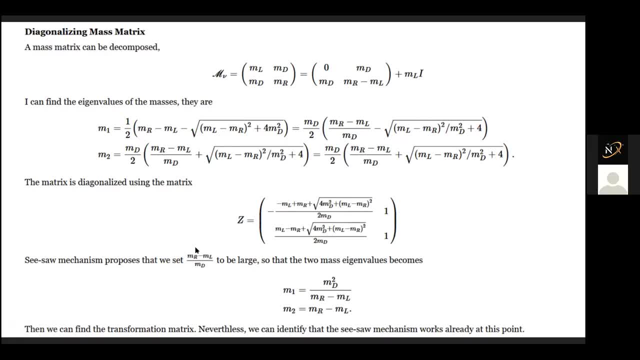 Okay, This would be lambda plus and this would be the lambda minus part. So the proposed MR minus ML by MD to be very large, as I said. So this would be B by M, would be very large. squared d divided by mr minus ml, you can see that this term would be very small. m1 is hilariously. 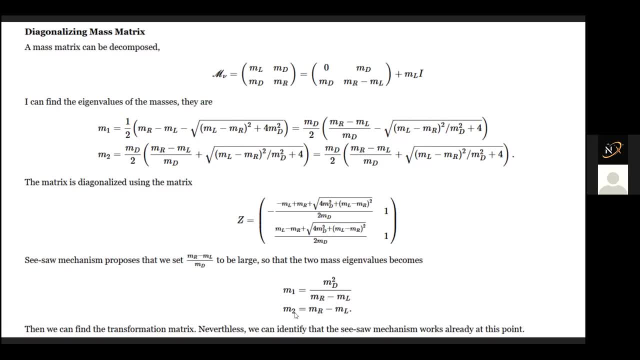 small, because mr minus ml is very big and m2 is almost equal to mr and that's going to be very massive. so we can see that. you know the seesaw mechanism works. so m2 is almost same as mr and m1 is almost same as ml, because if you subtract the two you're going to get mr minus ml because m1. 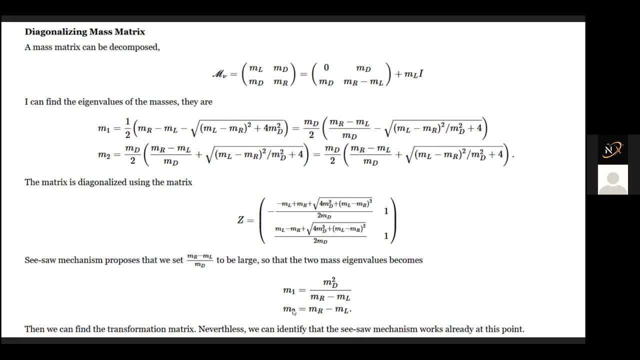 into m1. into m2 has to be m squared, if you remember from that the whole reason of seesaw, and similarly for ml into mr. so we have m, approximately m1 is equal to ml and m2 is equal to mr. so we have the two eigenvalues of the two masses with a corresponding coherent theories. 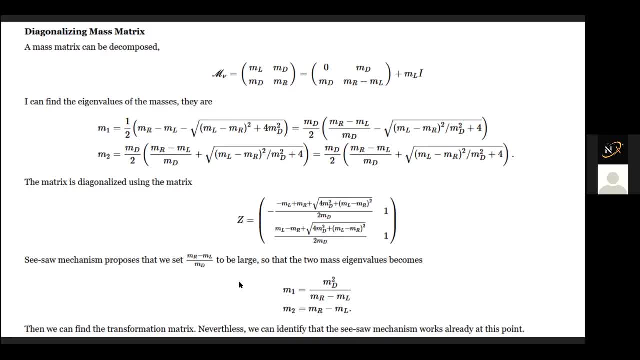 so this is a proposed thing. you know, m1 is what we've observed, the very low mass, and m2 is the sterile neutrinos. they're called sterile because we haven't seen them interact with anything, but they're sterile because they're sterile, because they're sterile, because they're. 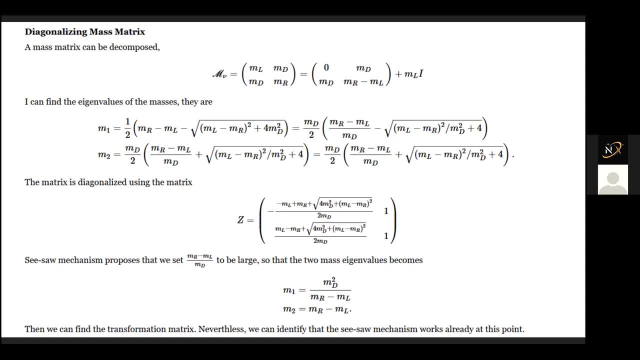 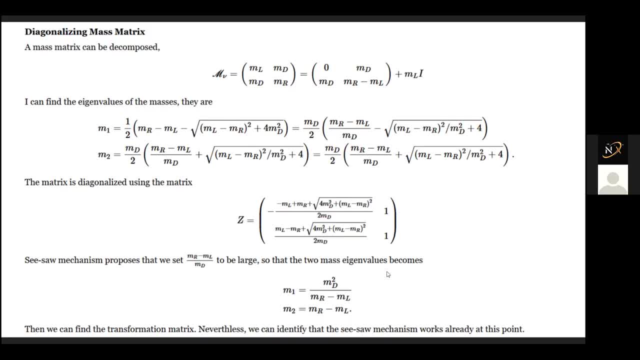 observational data. but this is a very uh looking forward like, it's a very forward thinking in the field of particle physics. even though this was done long ago, it's still a very, very viable theory till date. so we spoke about some- you know, uh, inconsistencies. all you know, all of these are 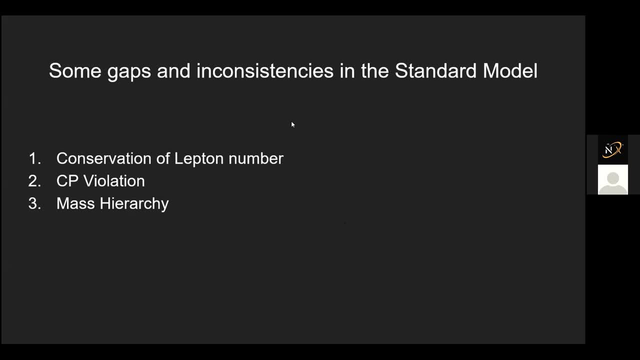 just changes to the standard model, but let's see what others you need to change. thanks to the major random mass and everything else, the conservation of the lepton number. this was first of all this came out to be as a empirical fact. this is already disproved by uh neutrino oscillations, as you know. 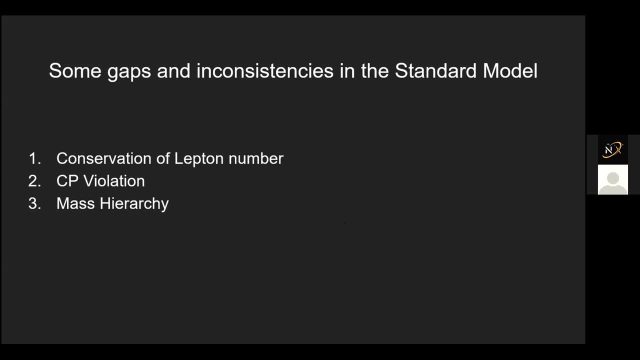 uh, people, uh, my teammates spoke about yesterday about leptonic mixing and everything. so you have changes. so the lepton number flavor is already uh violated, but you can see how this works even in the form of mass and um its extensions. so first we talk about the hamiltonian uh of the system. this would be: 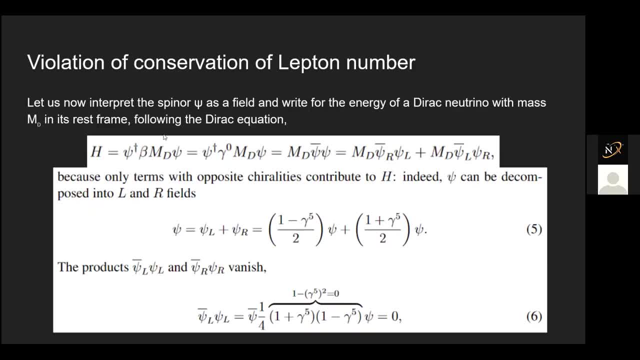 given by, you know, the dirac equation. um, i'm not going to derive this i i want to take it at face value because that's not the point of what i'm trying to do. so, in general, you can talk about the wave function to be, you know, as a superposition of the l and the r field, the majorana uh wave. 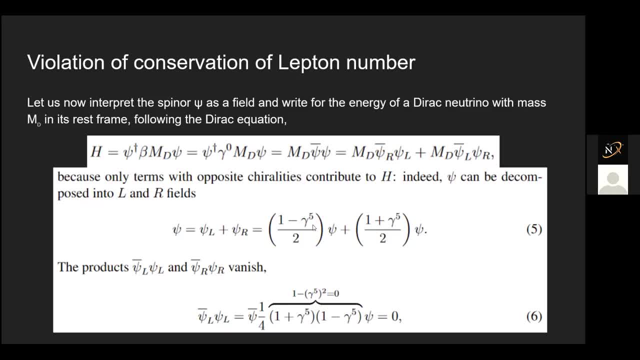 function, the spinner would be left as well as right chiral. so we know the- uh, we know the operators for left and right. right, there's one minus gamma phi by two and one plus gamma phi by two. so if you, if you do this and if you try to expand it into this form, you can see that whenever you. 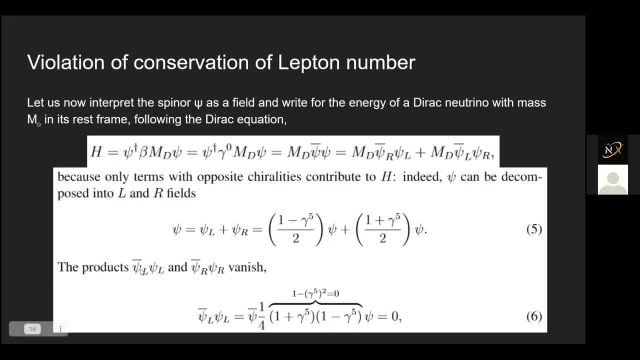 have, uh, a particle con, uh, anti-particle- like the bar would be anti-particle times its own- would vanish because you're going to have one minus gamma phi squared by two and that's going to be zero. so basically all terms with this is going to vanish when you try and open this. 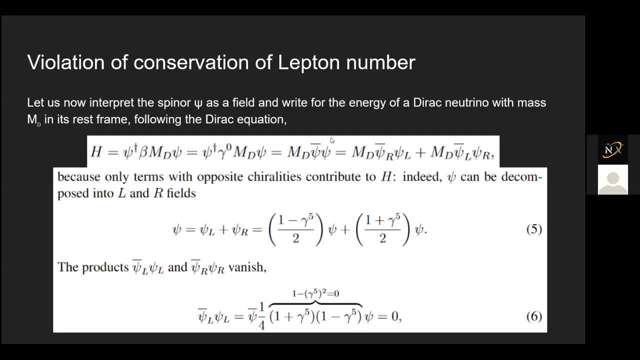 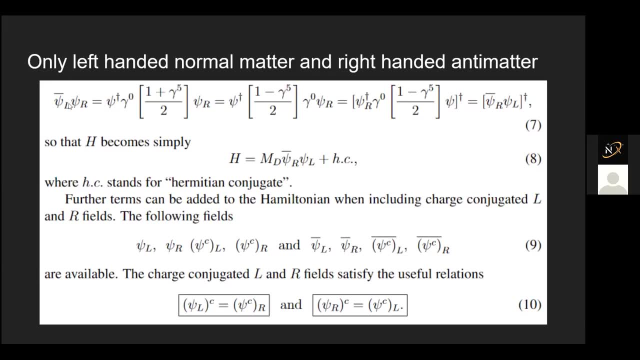 equation. so you're going to have only these terms remaining. so only left-handed normal matter and right-handed antimatter can exist. so because if you have a left-handed antimatter and normal right-handed matter, you can see that it is, it's after you go through the steps, it's going to be its own conjugate. it's going to sorry, it's. 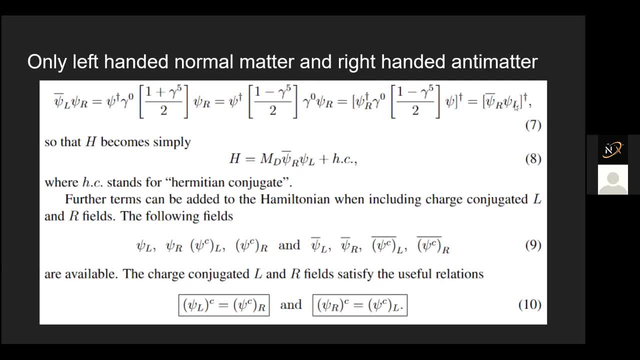 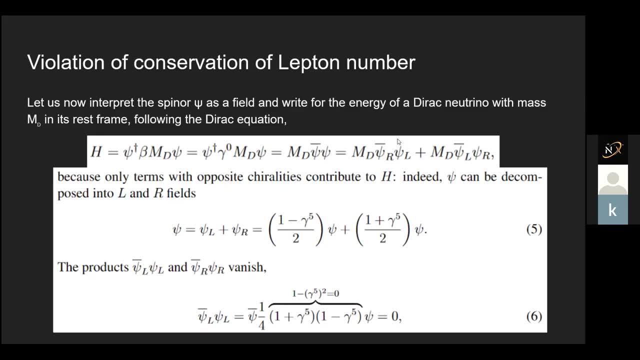 going to be the conjugate of right-handed uh anti-particle, as well as left-handed normal. you can write this the equation here, because we just proved that this is the conjugate of this, as this, plus its Hermitian conjugate, hc, is the Hermitian conjugate. we just showed that it's. 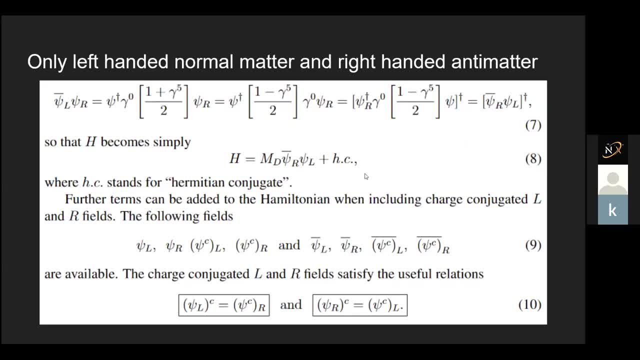 the Hermitian conjugate. it's it's easier to work with one term. it's. just seeing multiple terms everywhere would be uh kind of chaotic, uh. so you can add stuff. so the Hamiltonian, you can add it. you can add the charge conjugated part of the left as well as the r fields. so you're going to have 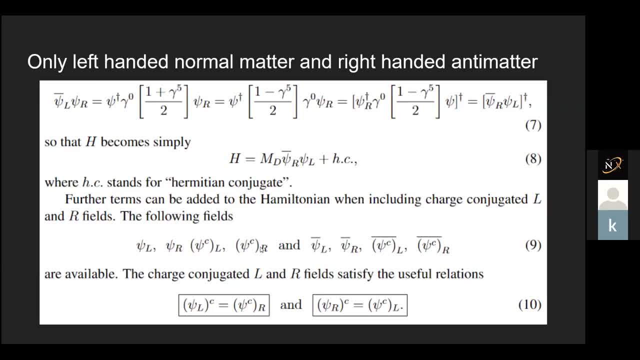 left, you're going to have right, you're going to have charge conjugated l you're going to have right, and then anti-l, anti-right, charge conjugated anti-left and charge conjugated anti-right. there's a whole bunch of probabilities, but some of them, thankfully, are, you know, cancelled or they. 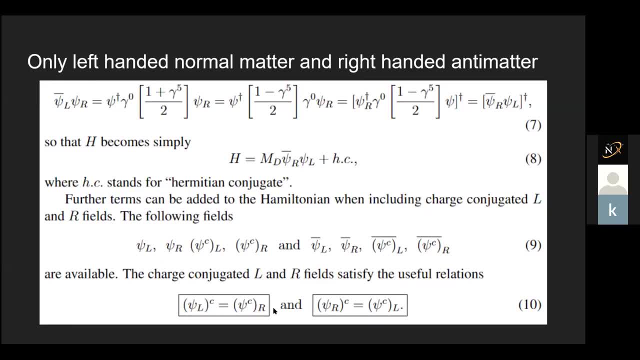 relate with each other because charge conjugated l is uh or l whole conjugate would be the conjugate times right meaning if you have a uh, left neutrino and if you try to conjugate it, if you try to get the antimatter, then you just have a conjugate in neutrino and you'll 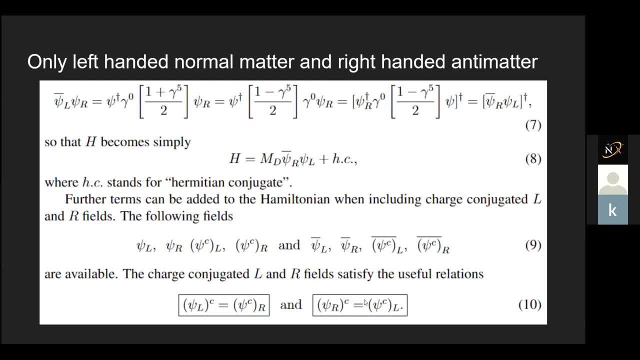 which is the antimatter, and you find that to be right-handed. so this is very, very useful relations. thanks to Majorana. this also explains why you have only left-handed- uh, you know, or you have right-handed- anti-particles to be the same mass as left-handed, because till now you just 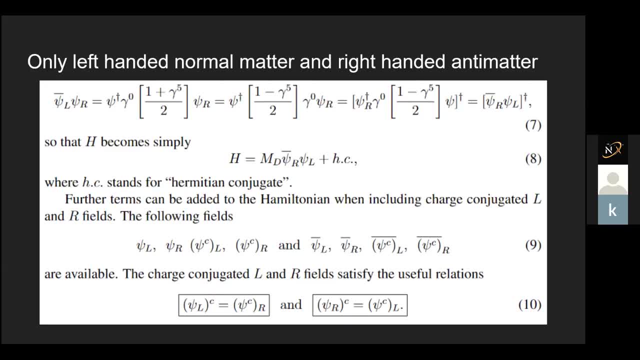 said like: look, Aditya, you just said you know left and right. uh, sorry matter, and neutrino and anti-neutrino of a Majorana is the same. so if you have left, how can it also have right? like won't that be very high mass? but no, this also answers that, which is very important. 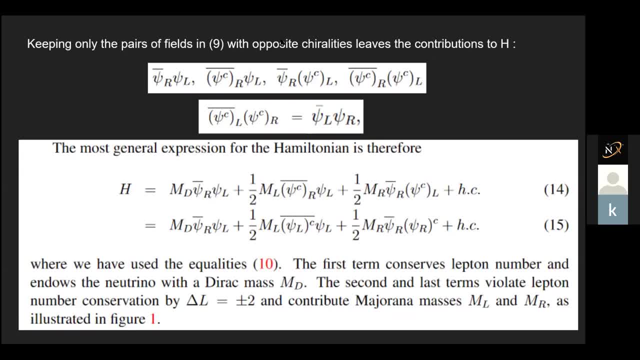 very cool. um, so, if you can keep only the ones with opposite chiralities, uh, from this equation, because we see that the same chirality comes vanish, keep the opposite terms, uh, you get this. and another useful relation would be this: uh, this is a pretty easy uh derivation term. they're going. 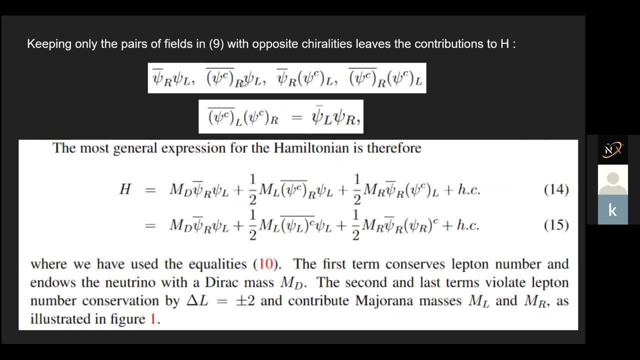 to do so now the Hamiltonian, if you add all these extra components left thanks to its. these are the Majorana field components. till now was just the Dirac part of it, because you see the MD part, but you add the Majorana part of it thanks to its. you know charge conjugate. so this is the equation okay. 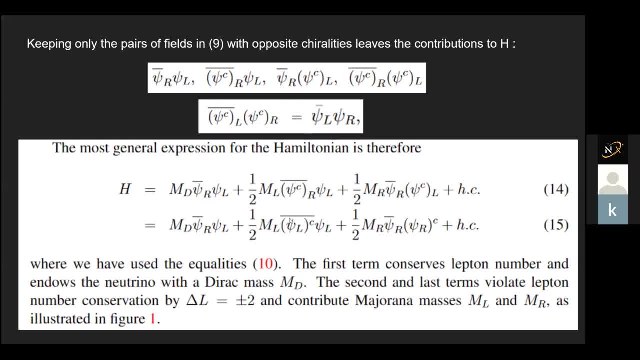 MD, uh plus half ML, times this: uh, psi L conjugate, uh, anti-neutrino, and psi L plus half MR, psi R, an anti right-handed, anti-neutrino, versus its conjugate plus. you know the Hermitian conjugate of each of these terms. so now we have used some of the relations and the first term conserves. 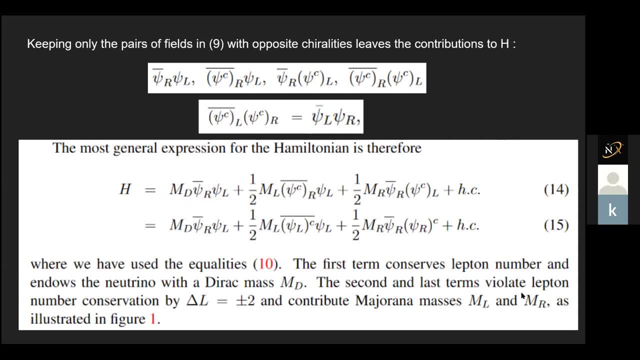 the lepton number here, MD is just MD, there is not much changing. but the second and the last term, uh, violate the uh lepton number because the Hamiltonian that we expressed before is just one particle. it would say just be an electron, but here you clearly have two other terms, which. 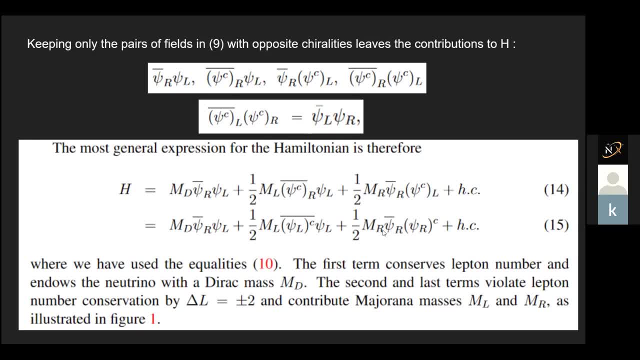 is, which is no related to this term, because they have separate masses. you know, the flavor of this does not matter. this could be electron left or electron muon tower, whatever. you have two more terms which each would have its own lepton flavor. uh, quantum number, and you're going to add 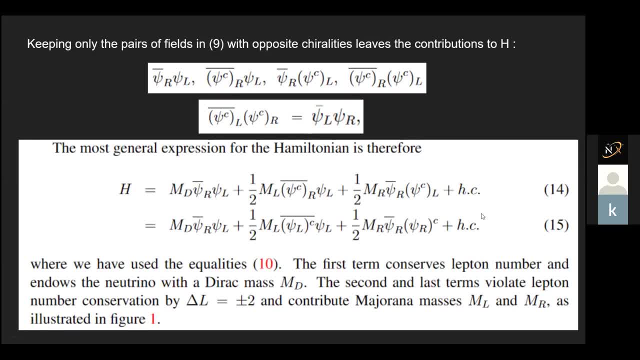 that to something that was already stable before, so it is going to be violated. it has to be violated. so lepton number conservation can also be violated in Majorana, as well as neutrino oscillations. uh, so what? what exactly does this imply? like? so what if you have a random mass term appearing? so 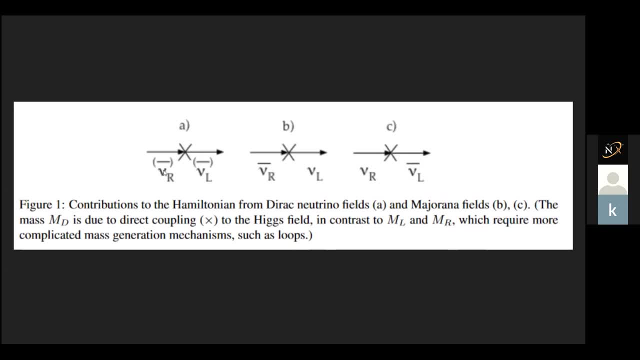 this means that in normal, if lepton number is conserved, if you have a right and a left neutrino, if you know one- uh, this is delving into quantum fields a little bit- so if you have a left or a night, uh, left or right neutrino or a left or right antenna, you know, if they annihilate they must give back their own. 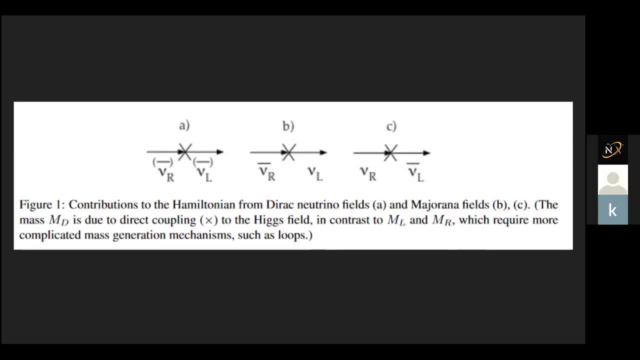 same thing, meaning if a right and left annihilate, you can either give right rise to a right and a left or an anti-right and an anti-left. but in Majorana you can have an anti-right, you know, annihilate and give rise to just a left or a right analogy and give rise to an anti-left. so there is a 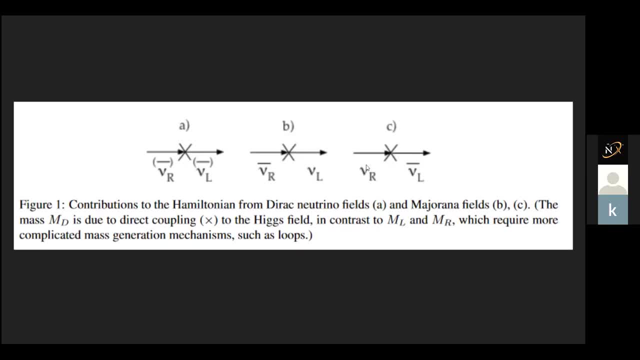 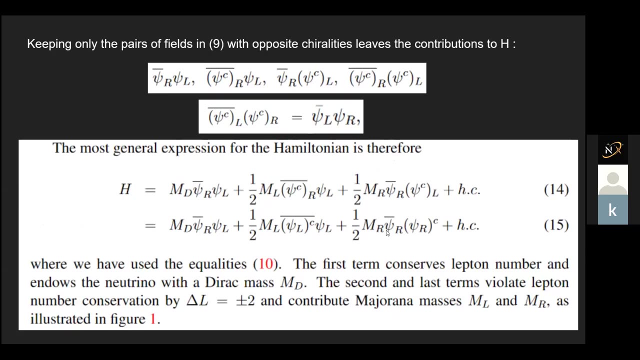 change in lepton number, because this would have plus one because it's normal matter and this would have minus one because it's anti-matter. so this, this shows the uh, uh, the violation of the lepton conservation number. this is what this term means, because you have the right appearing out of nowhere. 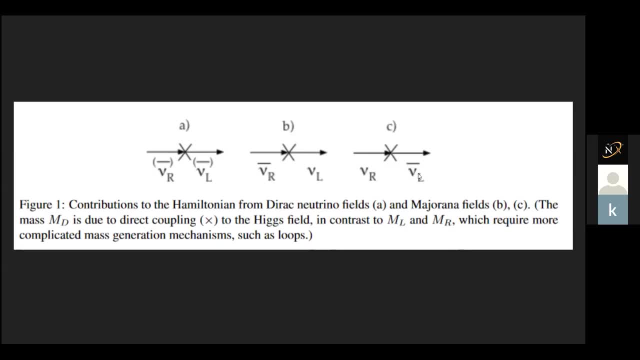 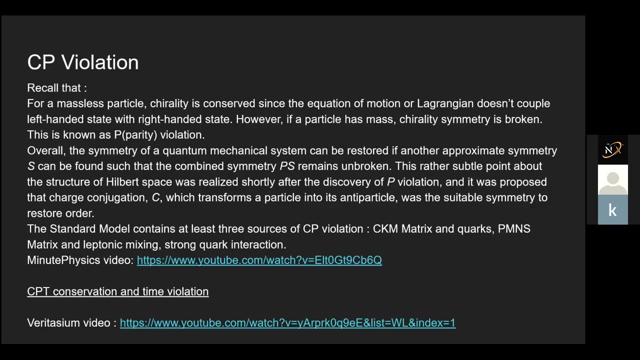 and that would be this: uh, you know, taken backwards because you have an anti-left and you're going to get that as a right. so that's one of the extensions of standard model that Majorana offers the uh, so the so observed lepton conservation violation. and then the second one was the charge. 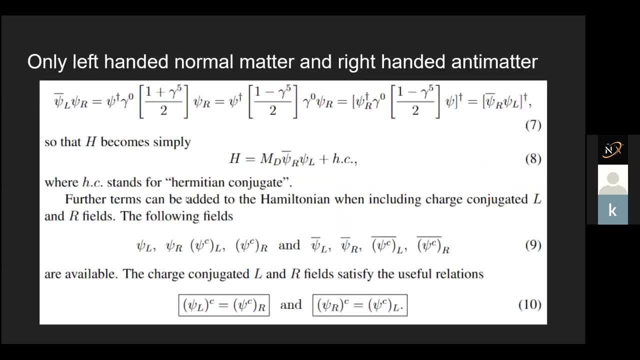 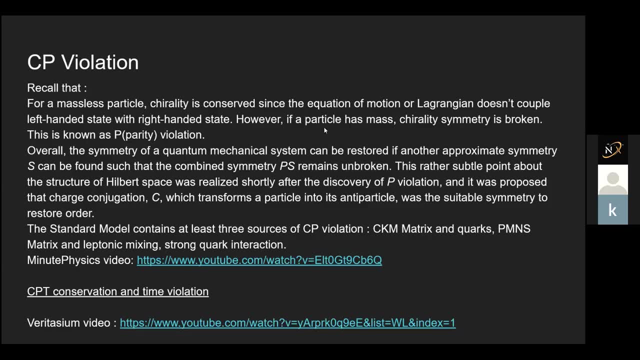 parity violation. uh, here we have the charge parallel and the mass hierarchy. so second one would be the charge, parity violation. so, uh, remember, I told in one of the key differences of Majorana that for a massless particle chirality is conserved, but if it has mass, then it's broken. and I told you, 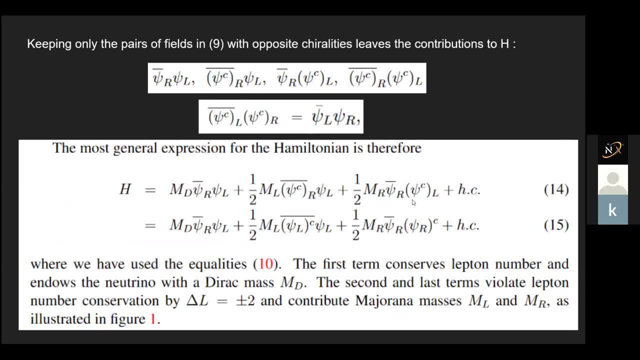 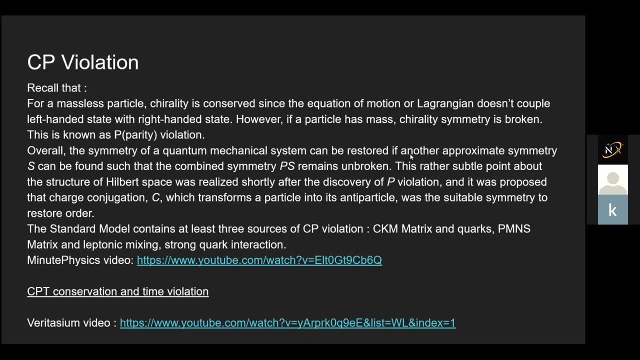 there's a reason. well, this is the reason you're going to have an extra right or a left term. whichever term you do have, it's going to violate the chirality or the parity. overall, the symmetry for quantum mechanical system can be restored if another approximate symmetry s can be found, such that the combined symmetry remains unbroken. 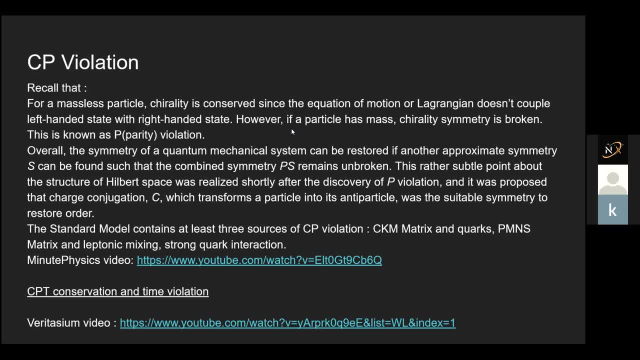 so they thought, uh, you know, if parity is broken, then maybe charge parity. uh, is what they came up with. maybe some other thing times parity would be, would still be conserved, because something has to be conserved. people could not be like, oh, this is broken. like you know, we try to find a very 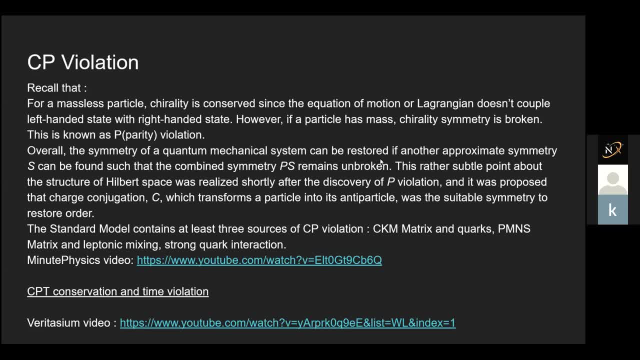 comprehensive, closed view of physics, and for that you need some quantity conserved. so this rather rather subtle point of Hilbert space was realized shortly after the discovery of the parity violation, uh, and it was proposed that the charge, conjugation C, which transforms a particle into its antiparticle, was the super, was the suitable symmetry. now, uh, this does, uh see. 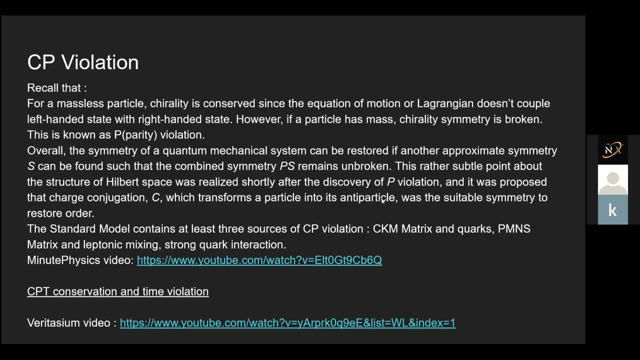 appear like very thorough. it explains all of the parity violations, but it gives rise to three new CPA violations. uh, one of them would be the CKM matrix and the course, which is very similar to the PMNS matrix, and electronic mixing. there's going to be mixing as well in the CKM matrix and even in the strong, strong quark interaction due to color. 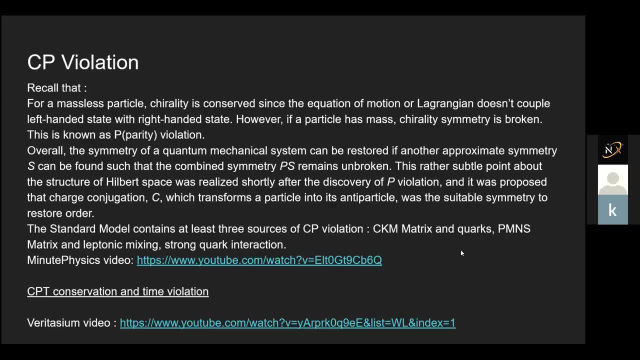 charges there. also, there's going to be a charge- parity violation- because the handedness and the color charge don't exactly go. now I want to show a video- a minute physics video- of the charge parity violation. he's going to explain better than I ever can and: um, okay, I think you guys cannot hear this. 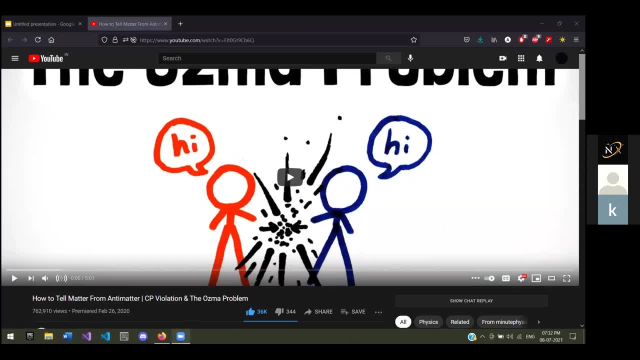 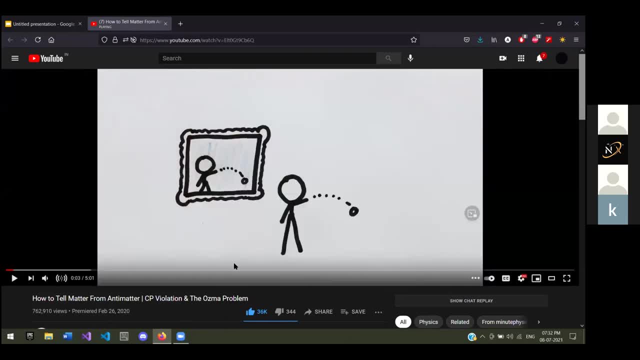 one second. I will just share the single app and not the entire screen. tell me, if you guys hear, uh, no on the on the, uh on the floating thing, the zoom floating thing, you'll have an option to share. uh, okay, share computer sound or something. share something. 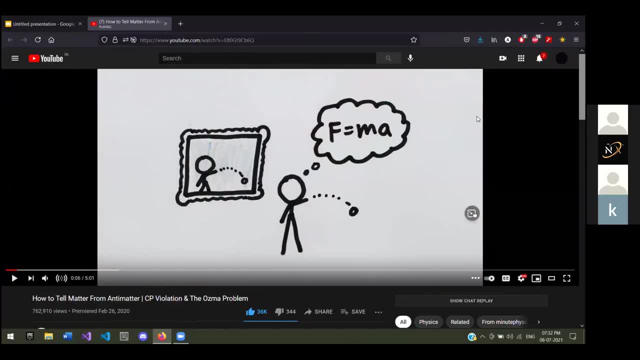 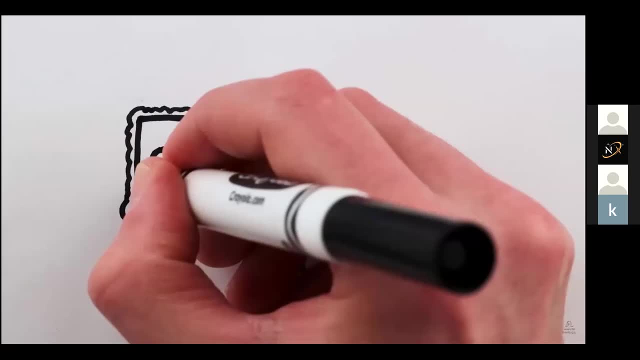 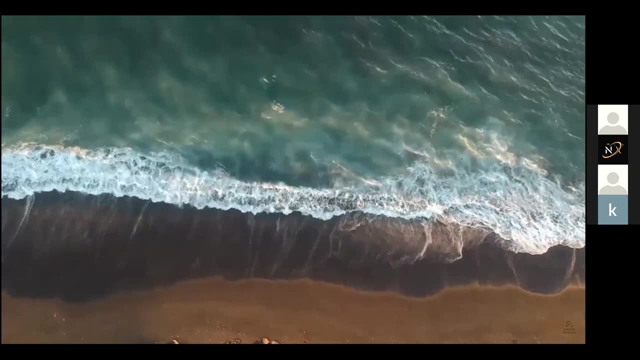 as they do normally, at least from a physics. yeah, we can help. yeah, we can. most everyday phenomena happen equivalently in a mirror clearer- as they do normally, at least from a physics perspective, Unlike when you play a video backwards in time, where it's pretty obvious that something 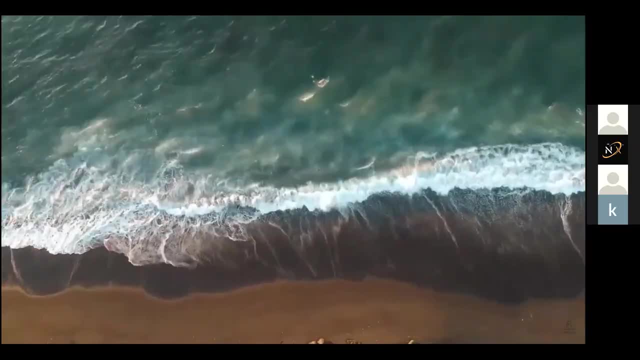 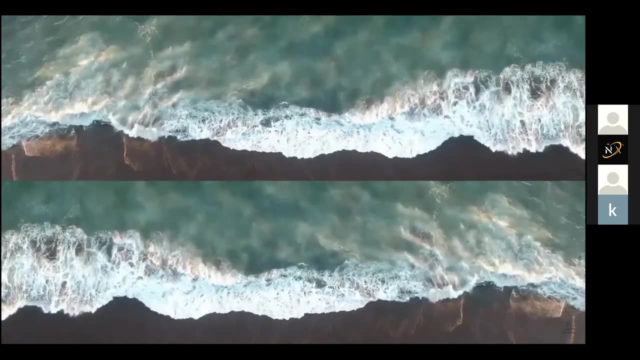 weird is going on. when, compared with a normal video, motion in a mirrored video still looks totally physically normal, just mirrored. In fact, without outside context, there's no way to tell which was the original and which was mirrored, which is why horizontally flopped shots are used in movies all the time. 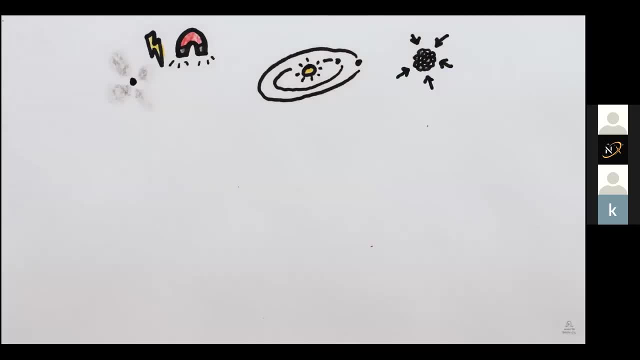 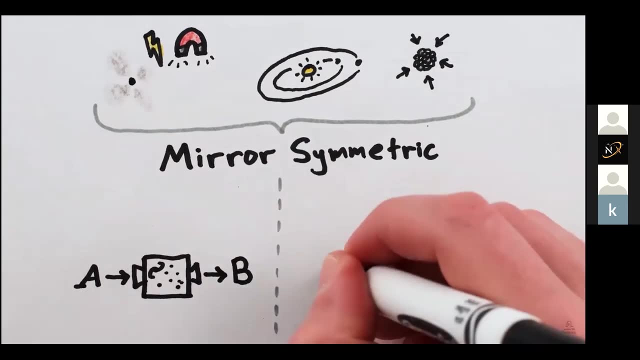 In fact, as far as we know, everything in the universe governed by electromagnetism and gravity and the strong nuclear force behaves this way. If you set up two experiments that are mirror images of one another, they'll produce results that look like mirror images of each other. 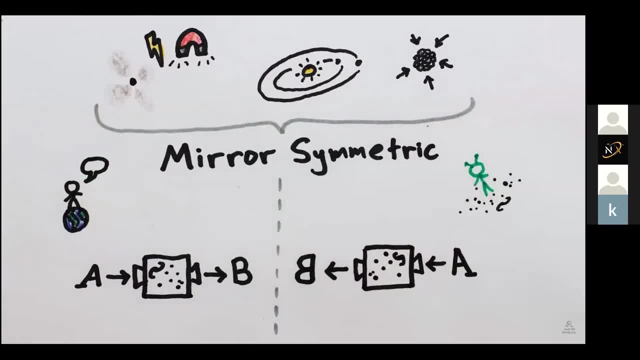 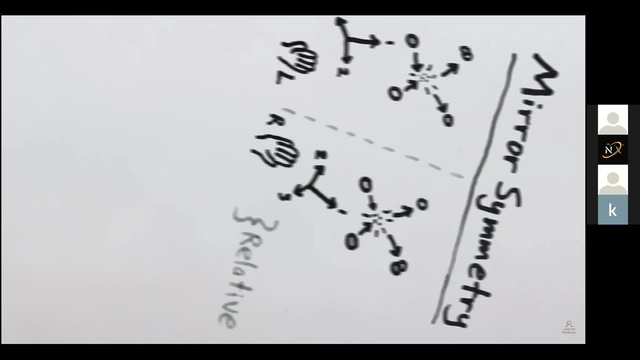 Which presents a problem if we ever need to communicate with aliens from afar. If all physics is mirror-symmetric, that would mean left-handed and right-handed are relative, just like up and down and forward and back. so if we were communicating with aliens and 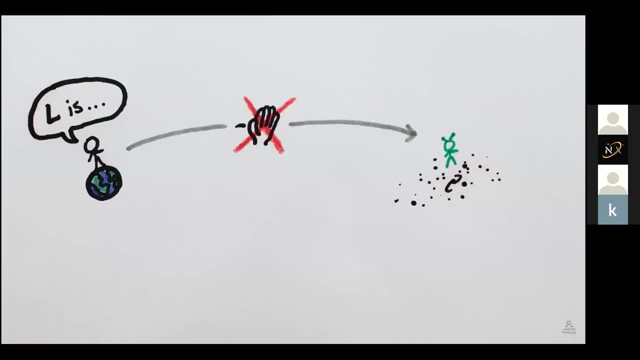 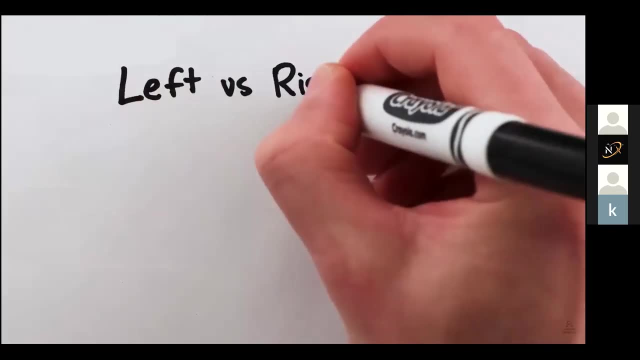 didn't have any shared reference objects, we'd have no way of explaining what we mean by left-handed and right-handed using physics. This left-right ambiguity is called the OSMA problem, And the distinction between left and right is important because Earth-based life mostly 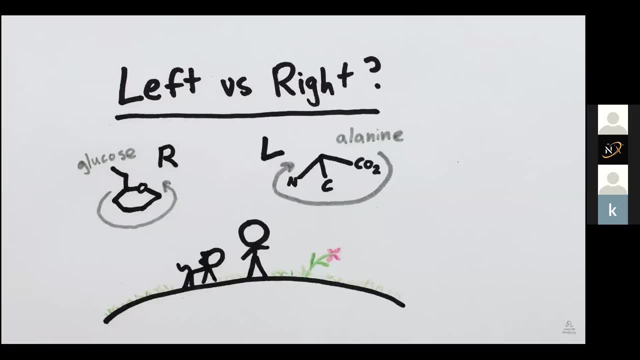 relies on sugars with right-handed symmetry and amino acids with left-handed symmetry. This isn't a physics constraint – it just as easily could have been the other way around – but the point is, the molecules in our food and our bodies do have a specific orientation. 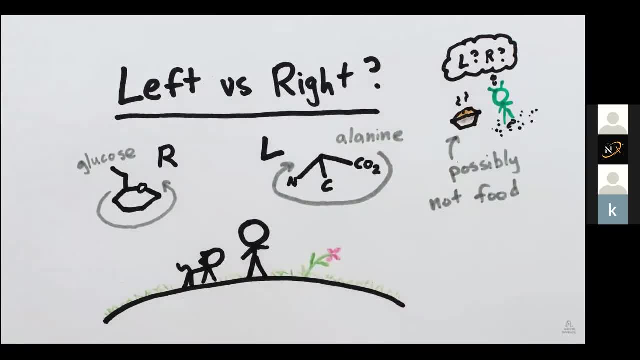 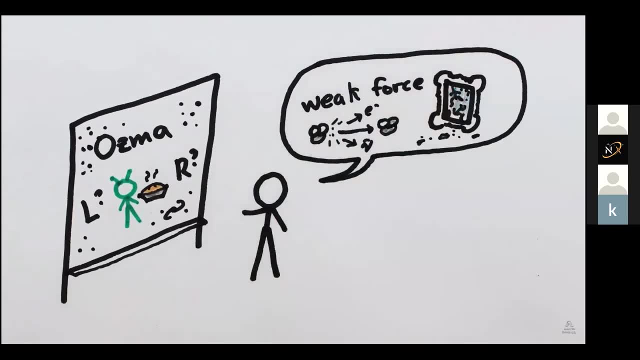 so not knowing left from right could impair intergalactic culinary relations. However, there is a solution. The weak nuclear force which governs the decay of subatomic particles doesn't always play nicely when mirrored. For example, When uranium nuclei beta decay, they emit mostly electrons spinning like left-handed. 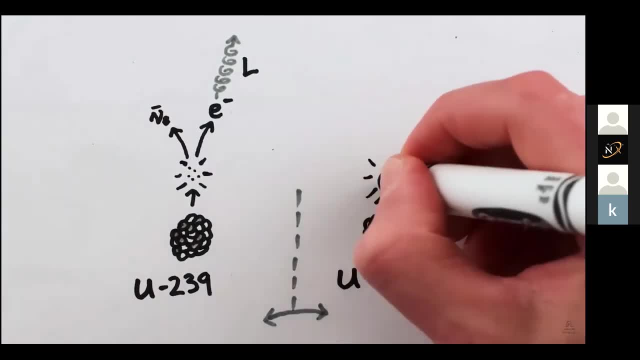 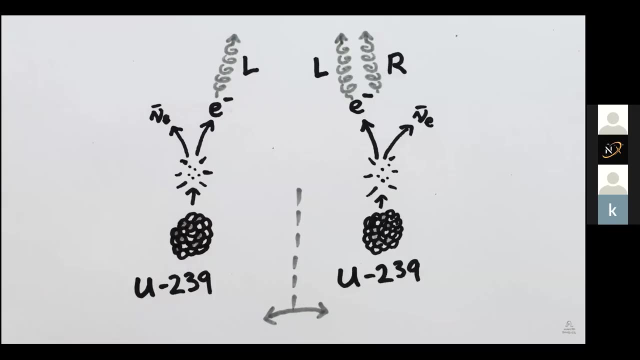 corkscrews. But if you perform the mirror image of the experiment using a mirror image uranium nucleus, the nucleus still emits electrons, spinning like left-handed corkscrews rather than right-handed as they would in a mirror. It turns out that in our universe the mirror image of a physical process doesn't always 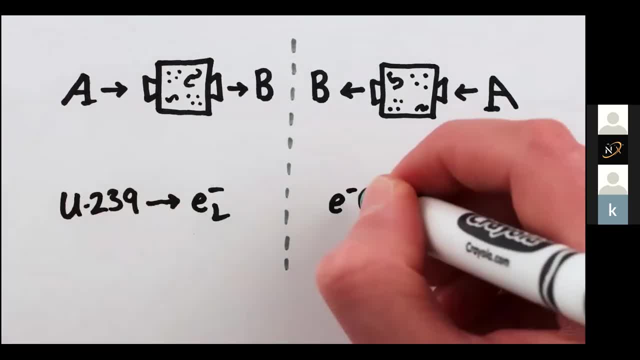 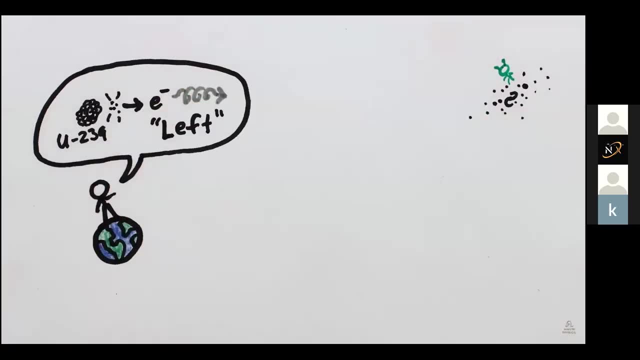 result in the mirror image of the outcome. Uranium always decays more into left-handed electrons, no matter how you look at it. So we could tell the aliens. you know how electrons spin when uranium decays. That direction is what we call left. 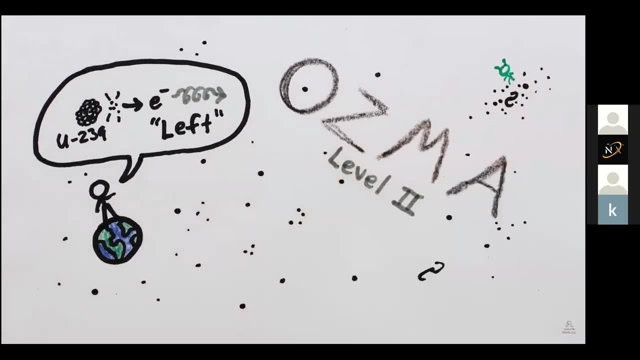 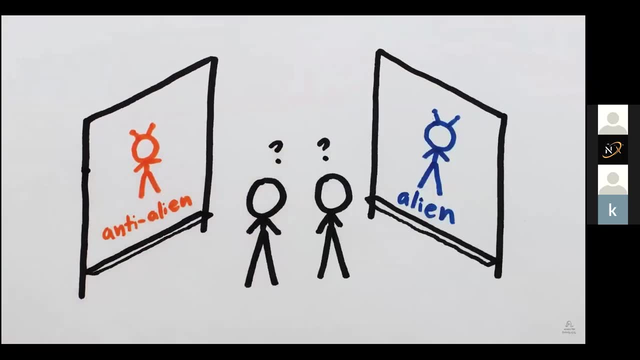 Which would solve the Osma problem, except our universe has a next-level osma problem up its sleeve, Because what if the distant aliens were made entirely of antimatter? I mean, in principle they could be and we wouldn't know. Antimatter interacting with itself behaves exactly like matter interacting with itself. 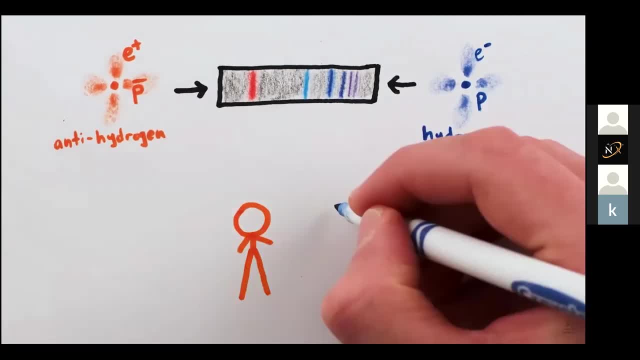 antihydrogen has the same atomic spectrum as hydrogen, and antimatter-u looks and behaves exactly like matter-u, until it interacts with matter. And here's the problem, While the matter-version of a uranium nucleus always decays into left-handed not-matter-u, 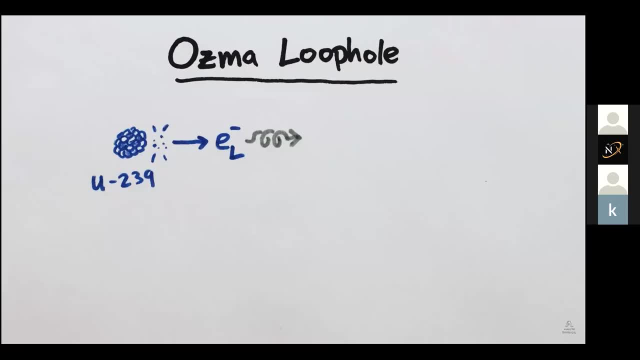 it's still not fully known to beurday. What is the problem? left-handed electrons- whether it's in a mirror or not, the antimatter version always decays into right-handed anti-electrons, whether it's in a mirror or not. 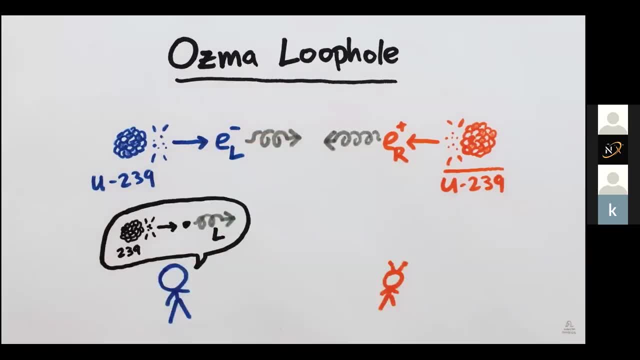 So if we told the aliens look at the beta decay of the nucleus with atomic weight 239, that's always the orientation we call left-handed- That would be wrong. For aliens made of antimatter it would in fact be what we call right-handed. 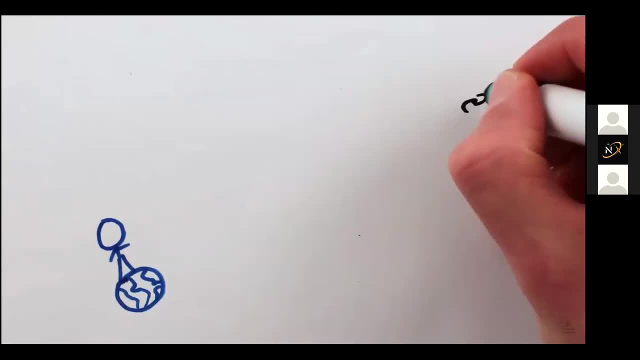 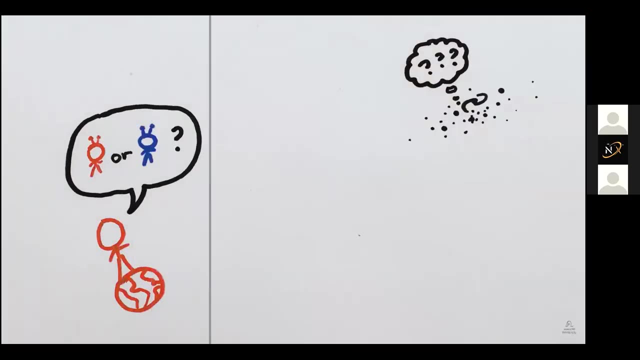 And you definitely don't want to shake either hand of an alien made of antimatter. So how can you figure out from afar whether or not a distant alien is made of antimatter? This is the OSMA problem, level 2. Essentially, antimatter is another kind of mirror we can hold up to the universe, which 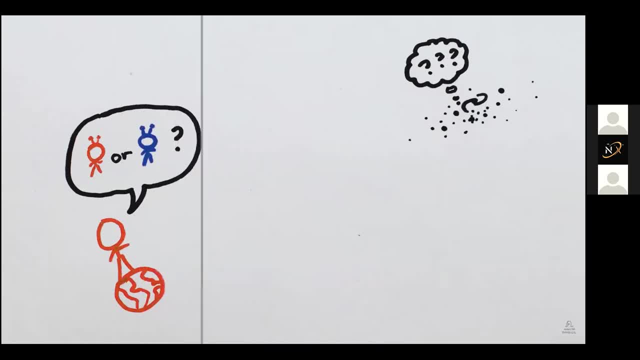 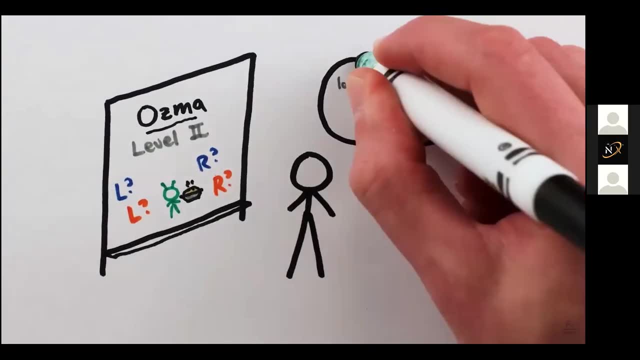 combined with the possibility of regular mirroring, means we can't use beta decay to define left versus right. But luckily there's a next-level solution, again thanks to the weak nuclear force. Enter the kaon, a fast-decaying subatomic particle. 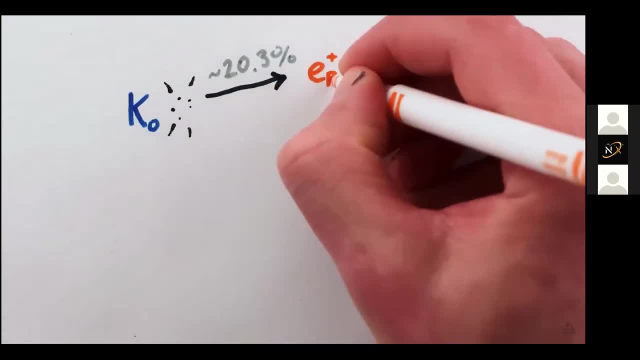 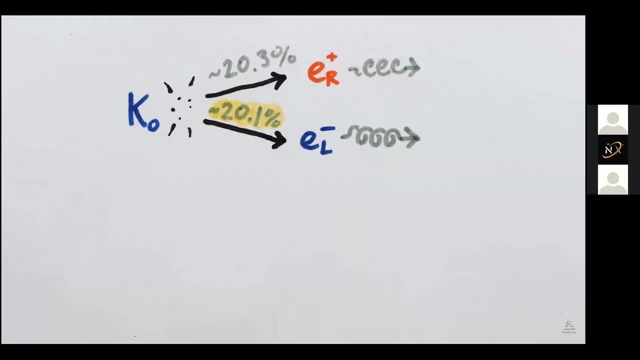 Whether they're mirrored or not. around 20.3% of the time, kaons decay into right-handed anti-electrons, while around 20.1% of the time- slightly less often- they decay into left-handed electrons, And the key is…. 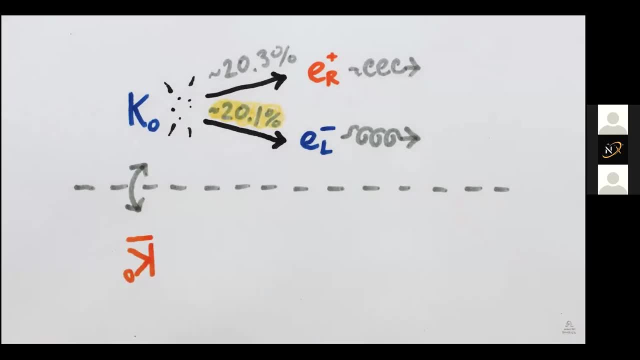 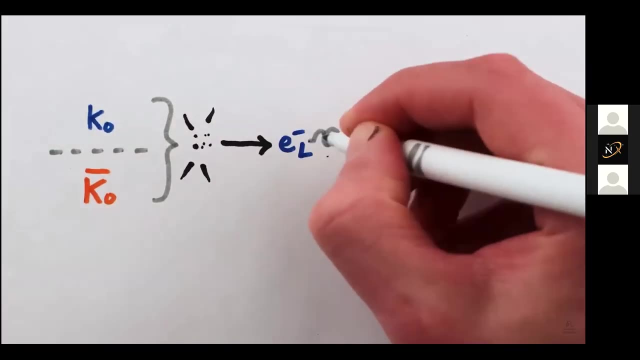 is this. If you instead take antimatter kaons, whether mirrored or not, they still decay slightly less often into left-handed electrons rather than right-handed anti-electrons, as you might expect. That is normal. kaons and anti-kaons both decay less often. 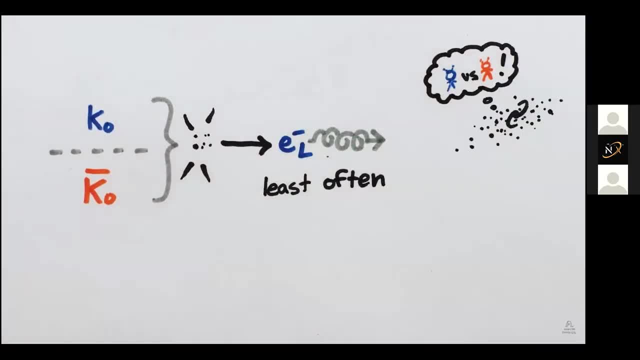 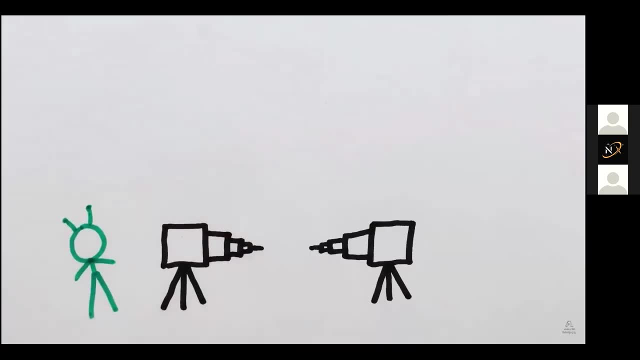 into left-handed electrons, And this is how distant aliens could figure out if they're made of matter or antimatter, and whether or not they're using the same concept of left and right as we are. Simply build a particle accelerator and look at the decays of neutral kaons. 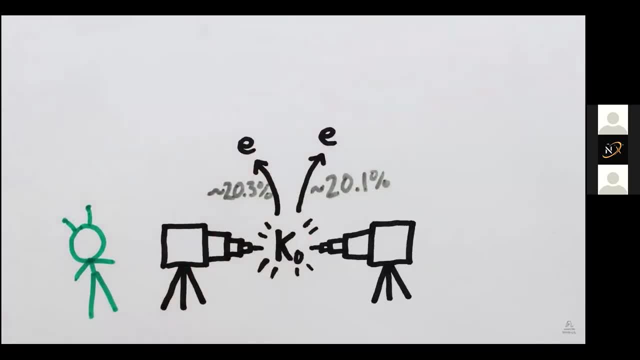 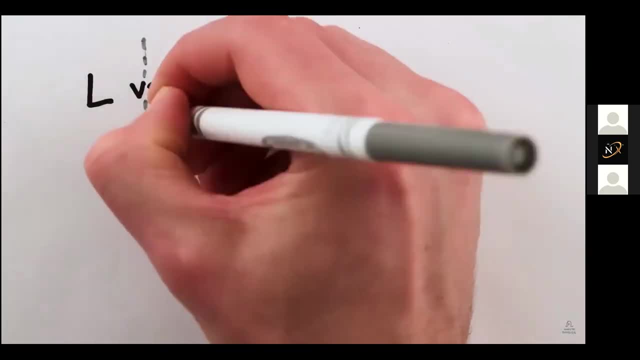 The electron-like thing that they decay into slightly less frequently is made of what we call matter, and it'll be moving in what we call a left-handed way. The universe doesn't distinguish between left and right or matter and antimatter for electromagnetism, for gravity and for the strong nuclear force. 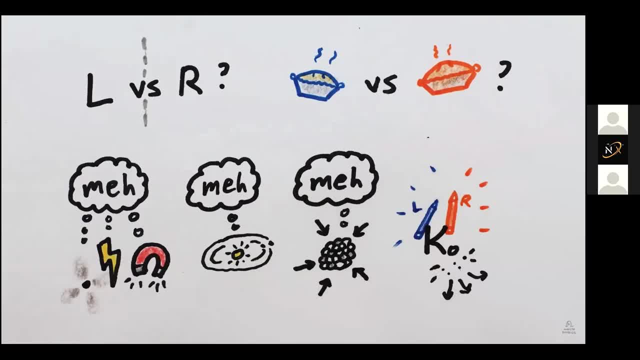 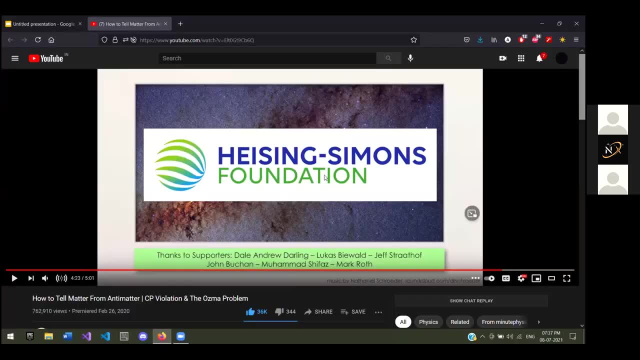 But for some reason the weak force allows us to tell the difference. This video was made with the generous support of the High School of Science and the University of Chicago. Uh, okay, So I hope you guys make that. Thank you, Bye. 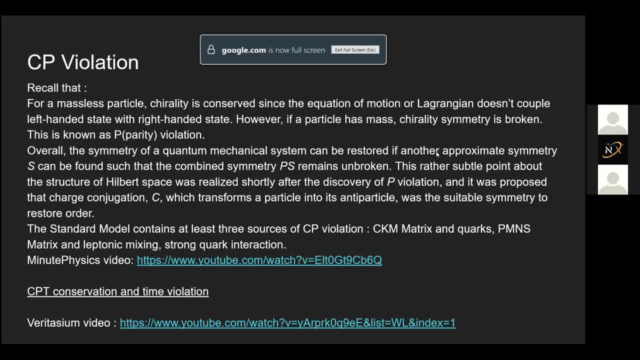 So that would be the charge parity violation because, as he said, they are able to distinguish it in a mirror. so would you not call that violated? But there is another thing, a deeper sense of a conservation law called the charge parity time conservation law. 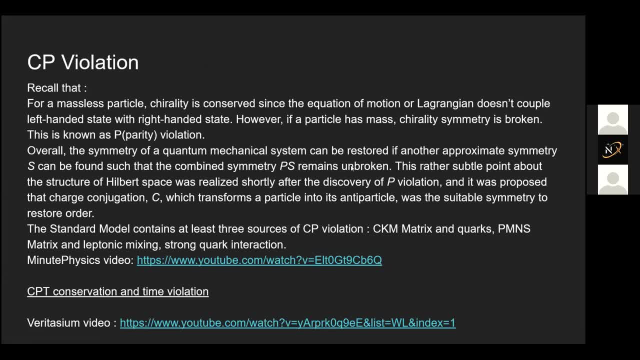 This is equivalent to adding another thing, like how you add a charge onto parity, you add time onto a charge parity, and this so far hasn't been proven wrong at all. But uh, so if CP is violated and CPT is not violated, this is equivalent to saying the: 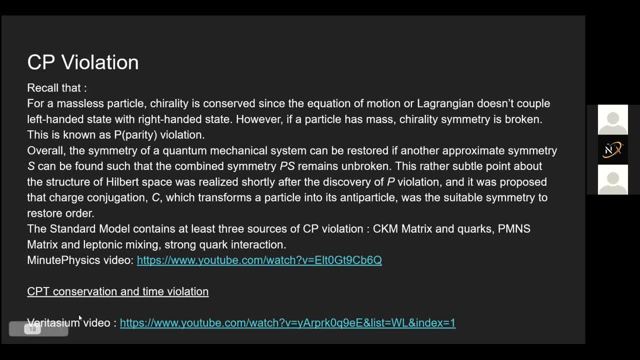 time has been violated, right, And in fact there's a very cool video made by Veritasium on that and the link is here. I will send this later to you guys. It's a good watch, but it's kind of long. it's like 10 minutes and uh, that's uh. 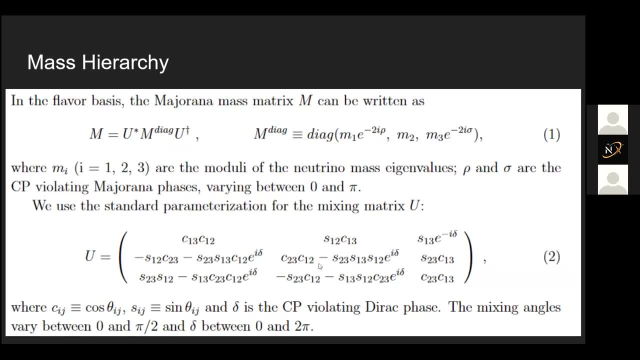 I think this talk has gone on for long enough. Uh, Now, the third thing of the standard model that it fails to answer is the mass hierarchy. Now, the mass hierarchy is essentially the way you arrange the mass of the neutrinos, the three masses, the three mass eigenstates: one, two and three. 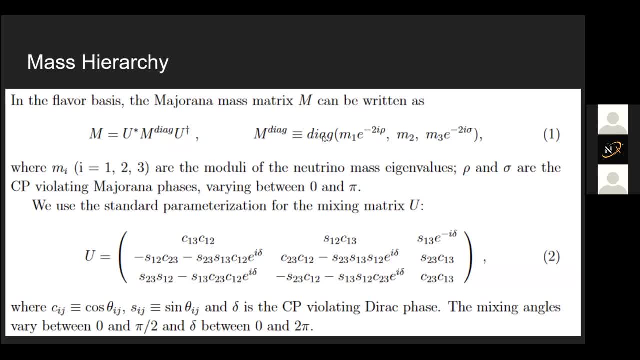 So this is the major and the mass matrix. I'm not going to derive this, uh, but yeah, just trust me. it is The moduli of the neutrino mass eigenvalues, the rho and the sigma. other sigmas, uh, not. 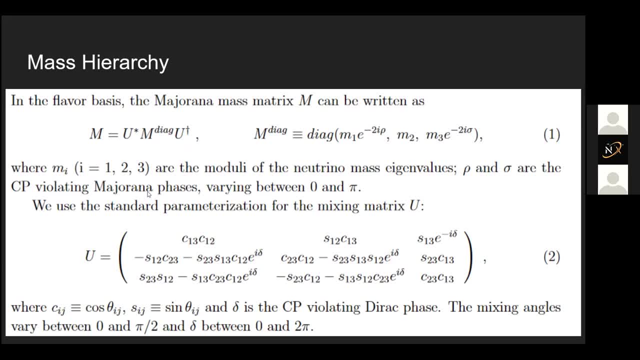 what we use for the gamma matrices. this is a different one. This is the Cp violating Majorana phases. As I said, the Cp violations will have phases- uh, depending on the violation angle, And there are two different angles and uh in the Majorana uh system and those are. 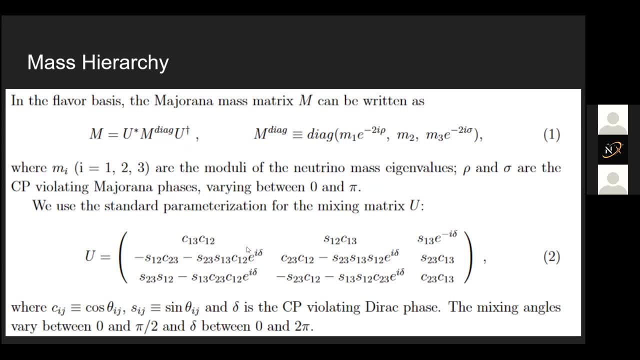 the sigma, those are the rho and the sigma. Uh, that you assume basically, you assume M, M2 to be like a standard relative mass and you try to get the other two masses, uh, in the form of expressing, in the form of violation. 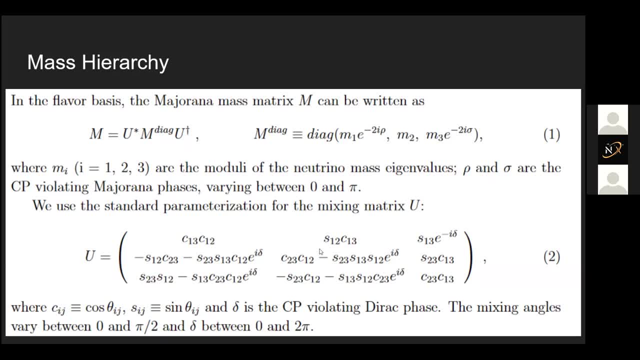 of the first one And, as you know, as you saw from yesterday, Uh, From the leptonic, uh, mixing this, this is the mixing matrix, this is the PMS matrix. Uh, the C would be the cost and S would be the sign, and delta is the Dirac phase. 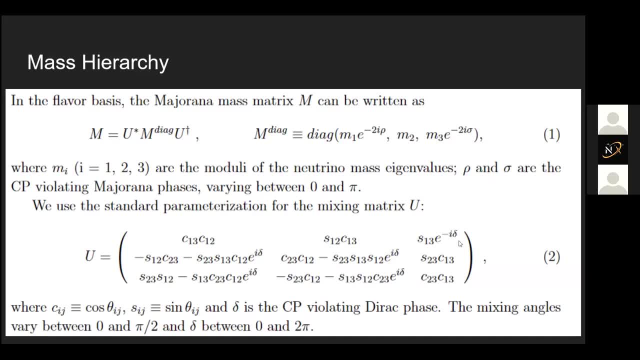 You know, standard model also causes Cp violation and Dirac started with a delta but Majorana really got up with it with rho as well as sigma, you need three uh masses, three factors or phases for like three violations Uh. so we consider the mass of and the mixing pattern which explains the atmospheric neutrino. 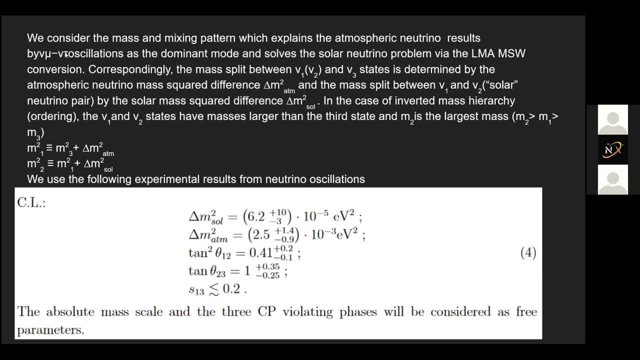 results: uh by uh the V nu, Uh the V nu to V uh tau oscillations as the dominant mode and solves the solar neutrino problem. Um, this is a different conversion, which I'm not entirely sure of either, but basically, 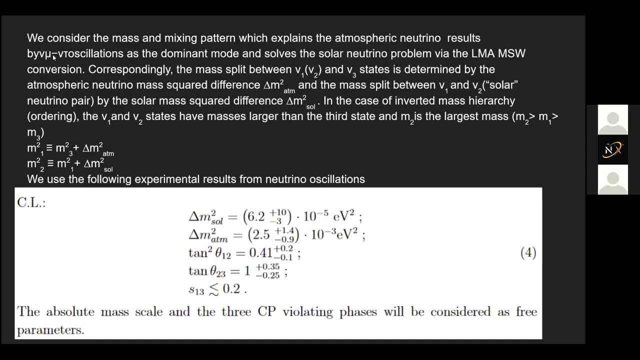 it assumes V. sorry for the formatting It. it assumes uh. mu muon to tau. neutrino conversions corresponding to the mass split between the uh, V1, which could also be two and three states, is determined by the atmospheric neutrino mass difference. because we know that, uh, you know, neutrino, uh, the atmosphere. 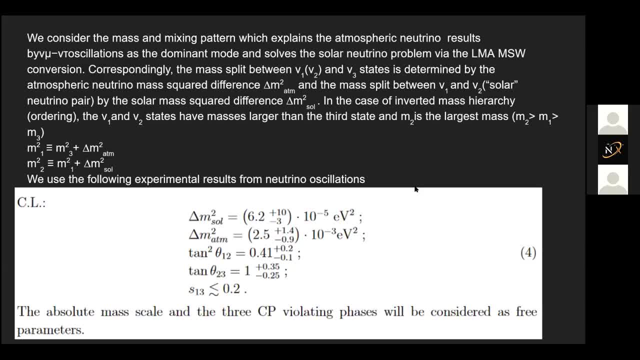 gives rise to two different neutrinos, As in a neutrino that mixes between two flavors and similarly a solar that mixes between two flavors. So by convention we call the solar mixing as one and two, because that's where we first got it. 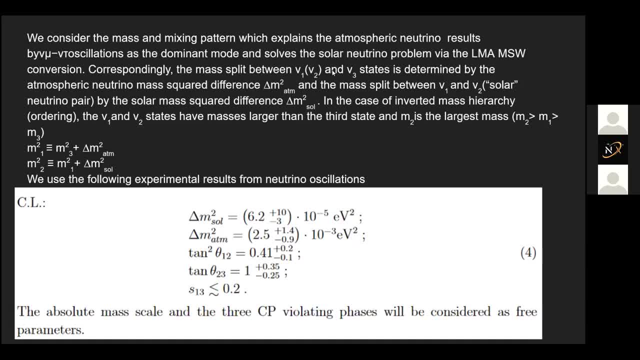 And the atmospheric mixing. we've observed that one of them, uh, one of the mixing phases, is similar to one of the solar phases, So it could be mu one or mu two. but the third, uh, another mass, I didn't say it's completely. 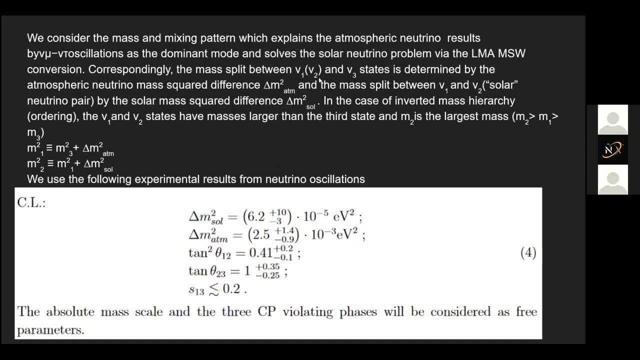 different, So this has to be three. This is why you don't exactly know which one is the first one and which one was the second one, because you can at best calculate the squares of the masses. the difference in the squares of the masses. 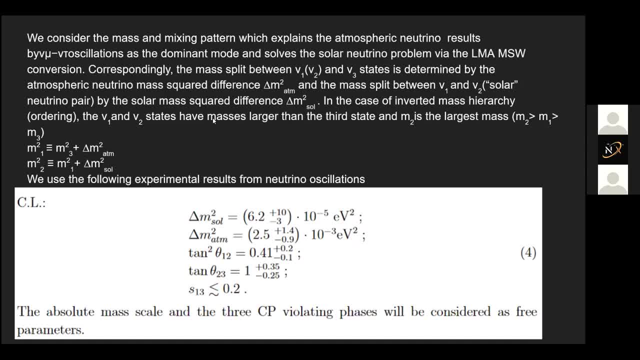 You can only calculate Delta M squared and Delta Sol squared. You can't get the exact M1M2.. That's, that's the entire problem with uh, any sorts of mass uh theories related to neutrino, whether it be Majorana, whether it would be standard model, anything, nobody. 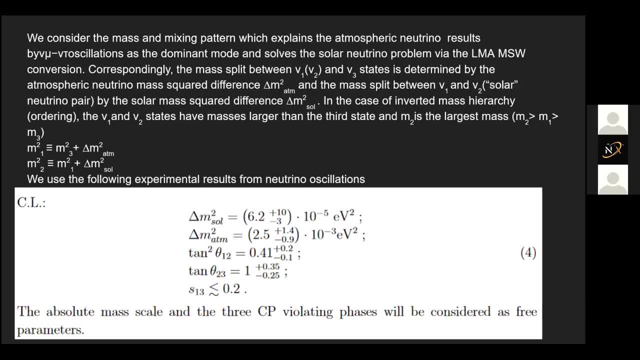 knows the exact mass eigenstates of a neutrino. It just doesn't exist. You can get only like an upper limit, uh, or a lower limit, Depends on the mass, Your limit, depending on which system you try to solve it with. but you can never get. 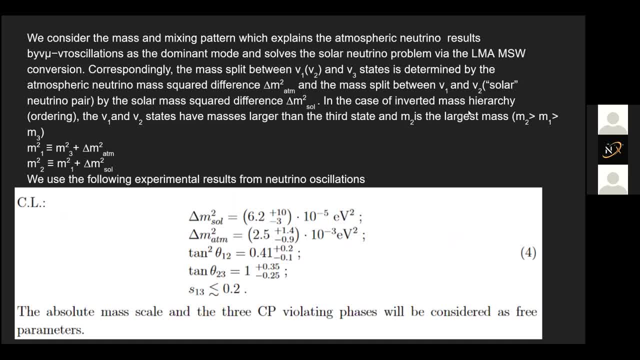 it And this is the main problem. So in a normal mass hierarchy you assume that the M mu three has the most mass. M three has the most mass, uh, and then M1M2, uh, as you would assume, to what one less than? 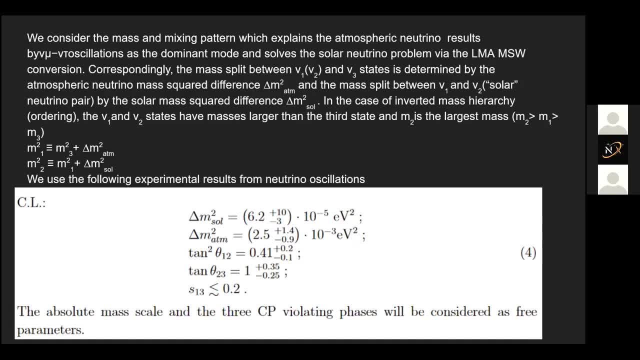 two, less than three, but in an inverted mass, since you don't know whether you know, M three is mu three is greater than or lesser than mu two or mu one, because you only have the Delta value, the change value, the difference value. 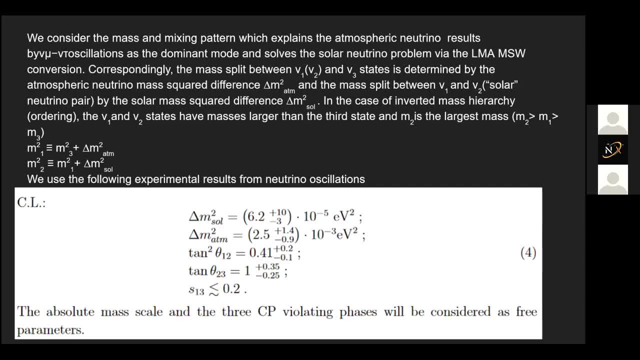 Uh, so you assume you know M two. First, we know that M two is greater than M one. This is the convention that we've taken by solar uh neutrino problems, without a doubt. So either M three is greater than M two or it's lesser than M one. that that's, that that's. 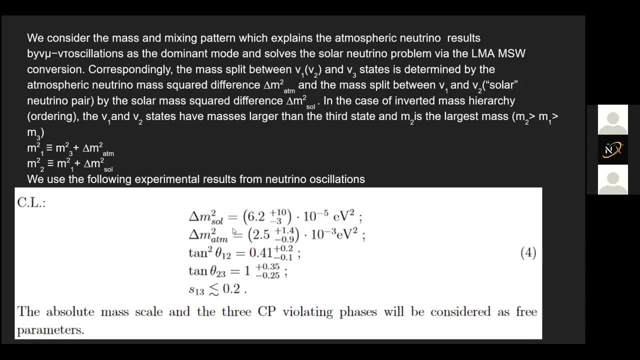 the only possible explanation for empty. So, if you see the results, I think this is from the Dune experiment and that these are the uh Delta masses that it would give you uh, and the mixing angles of one, two, two. 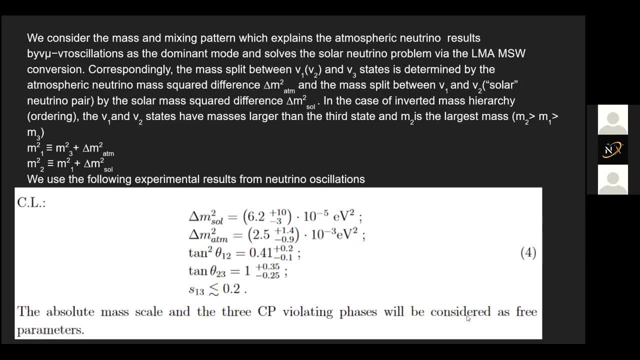 three, So the absolute mass scales and the three will be considered as free parameters. Remember how I told you: They're not constrained under uh anything's, they're just free. because, as of now, we don't know uh the exact mixing angles, because, Majorana, uh particles aren't even confirmed. 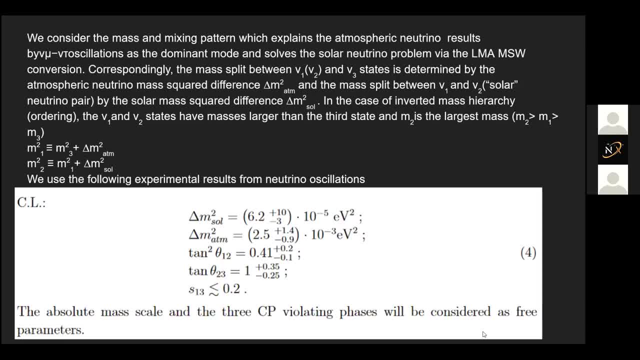 yet. So the phases of those, the row and the Sigma, are considered as free, whereas the Delta was, you know, very much real. it's in the PM and as matrix, the Delta part. Um, so yeah, uh, so this is a mass hierarchy. 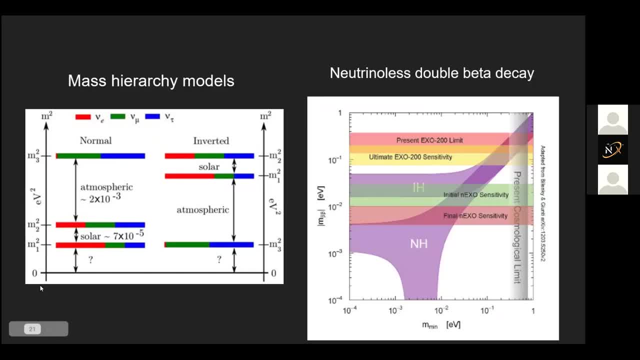 This would be the normal one that I said. So we don't know the exact mass, so we don't know the difference from zero to M one squared. So we know that the difference, the Delta M squared, is seven to 10 power minus five. 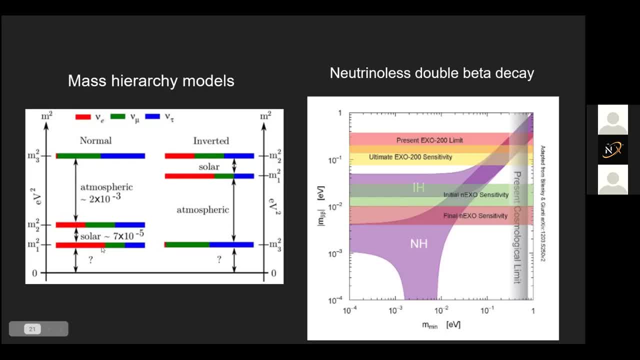 So we are assuming M one, M two squared minus M, one square would be seven to 10 power minus five, And we assume the difference between one of them, uh, of the solar and atmospheric, to be two to 10 minus three, the empty square. this is an electron volts squared, because 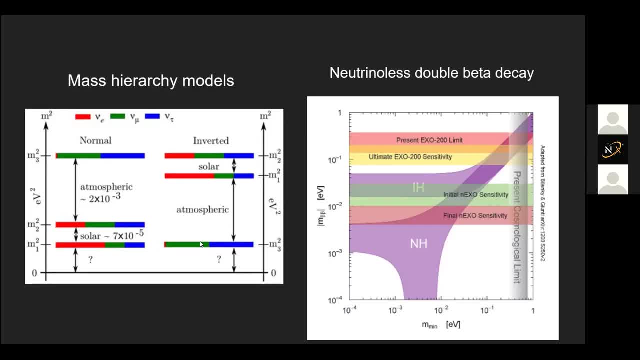 it's M squared, and M would be electron volts in natural units. Now, what if it were inverted? What is the atmospheric one? Very, very light. And this is what you would get instead. Then M three would be very low, and followed by M one, followed by M two. 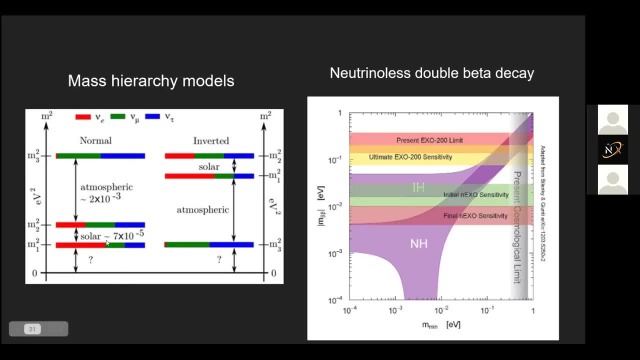 So this would be an inverted state, This would be a normal state And you can see that oscillations are very real, because the composite parts of M one would be a fraction of mu and mu tau, And for the atmospheric one it's mostly just new mu and new tau, but very little new electron. 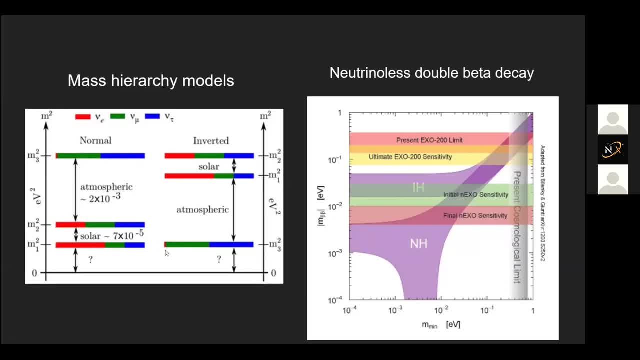 that has been proposed or detected. So how would you differentiate between them? Like I mean, look you, look at your detector and you say, oh well, okay, this is uh M one. for all we know it could be from solar. 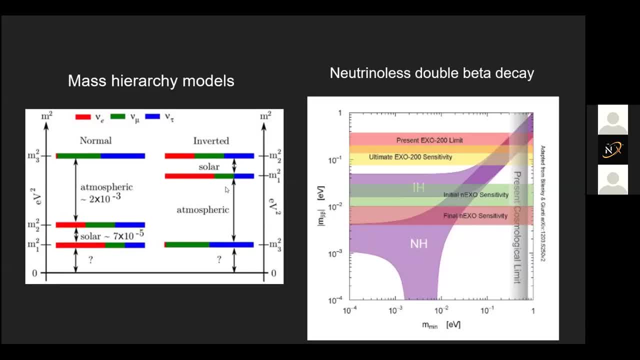 It could be from um atmosphere. It could be high mass, It could be low mass. You, you, it's a very vague thing. So one way on trying to find out, at least you know, if not the absolute value, at least. 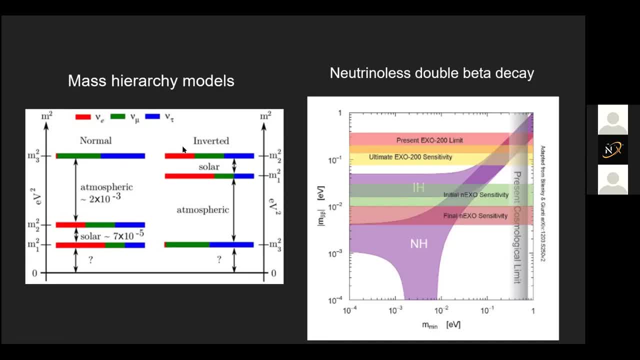 which is the correct model. we have two models: the normal and inverted. This is just a convention. This could have been normal for all we know, but since we first did get solar and then we put atmosphere on top of that, we take this as convention to be normal and the other 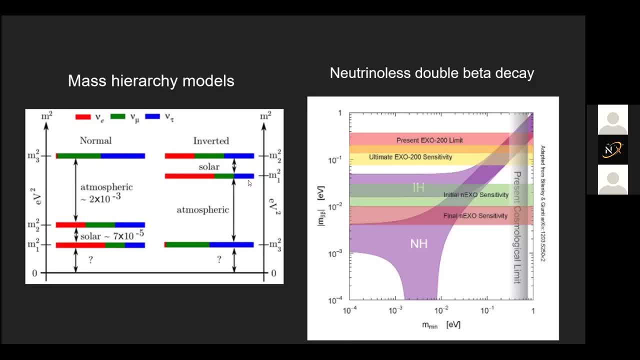 one is inverted. Now we put a function to Bogdan which is just uh low mass. But that professionals say is it's only variable, which are also a related function. What happens when B and M are related to the outside of the put? so for instance, we gave 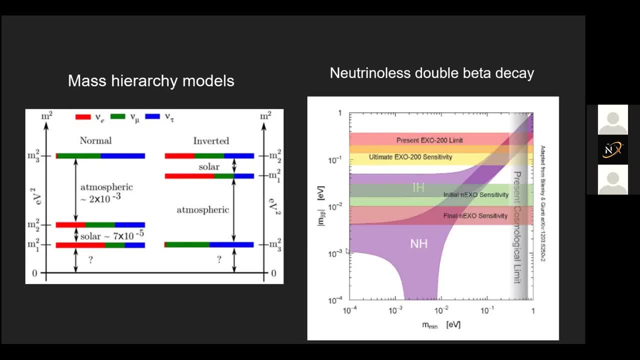 this bp. So B was equality. This is just a prediction. Okay, then we can say that the lightest neutrino out of that, meaning if it were atmospheric than m1- uh sorry, if it were atmospheric than m3 and if it were solar m1, then that would lie in this range. 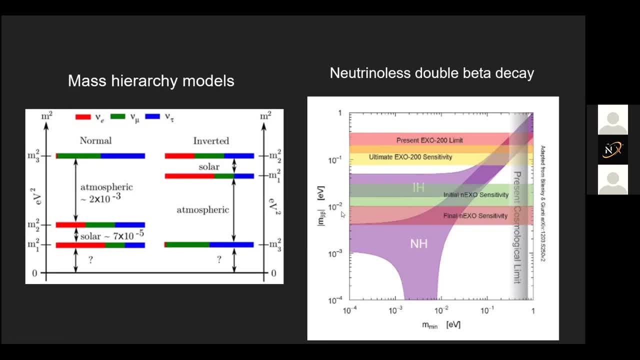 and if it were, uh, you know any heavier than this, if it was in the mass of this, then it would be an inverted- uh, head should be hierarchy. it would be in the inverted hierarchy. so a normal hierarchy is what we predicted. that would be like. you know this? uh, the graph would go like this, but an. 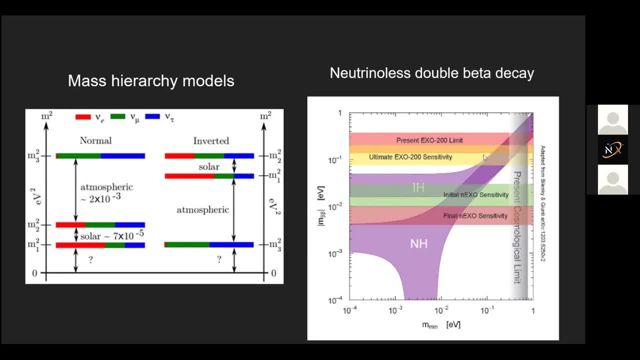 inverted one would go like this: it goes up this way: uh, you, you know that if it's inverted you you still don't get a lighter, you know like a lower mass limit for the thing at all. so this is why they say there's a specific mass limit for normal hierarchy, but not for inverted hierarchy. so 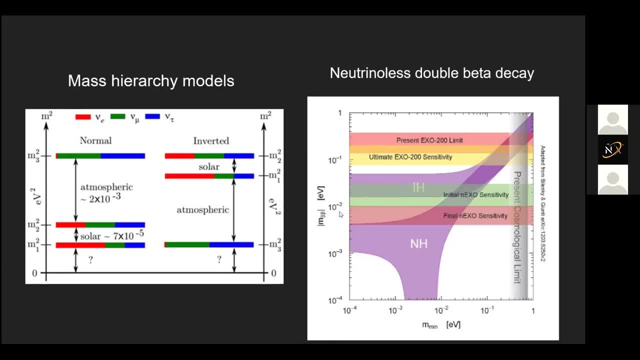 a newt observing a neutrino less but double beta decay would give us so much more information, confirmation of our theories, verification and further information on how to go about trying to solve more problems, because if you have at least have the lower limit, you can try to get in major animas and estimate. 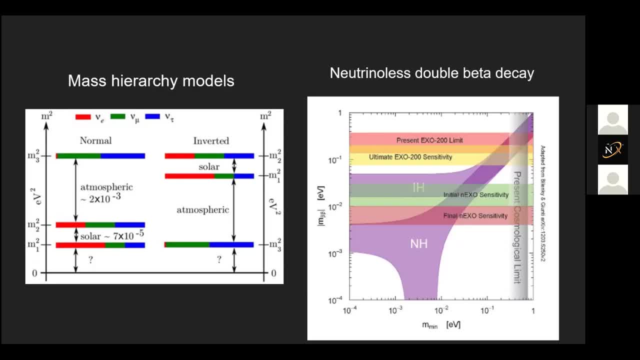 where the other upper limit right-handed counterpart would be, and try to search for that in that mass range. so a neutrino, but double beta decay is probably the most anticipated observation in neutrino physics. i would say. so this: uh, let's go. we've seen some. 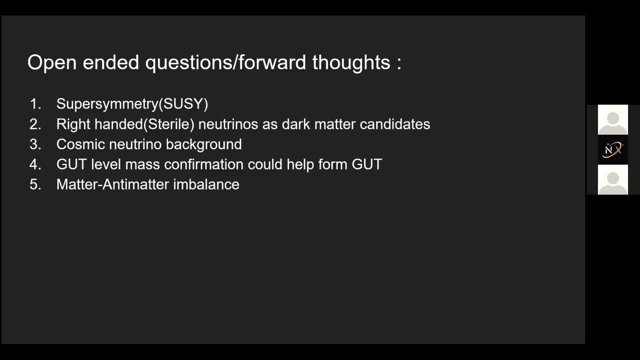 inconsistencies in sand model. we've seen how neutrons get mass, so now let's see about what we could think of if some of them were proved to be right or wrong. so one of them is supersymmetry. uh, so supersymmetry is a theory that i bet. 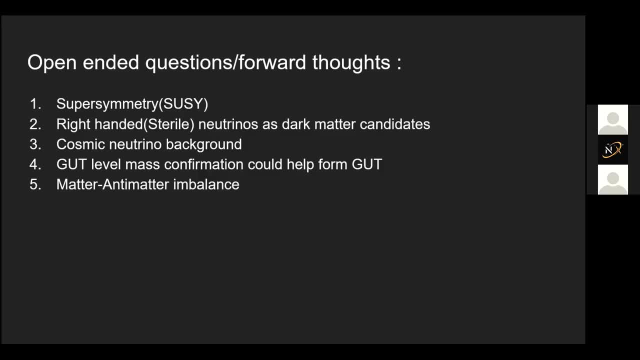 everyone here would have heard of: uh, it's. uh, it's a extension of the standard model. it's pro. it proposes that every particle in the standard model has a super part. partner like a lepton will have a slept on and uh like that. so the right-handed, you know, neutrino, could just be. 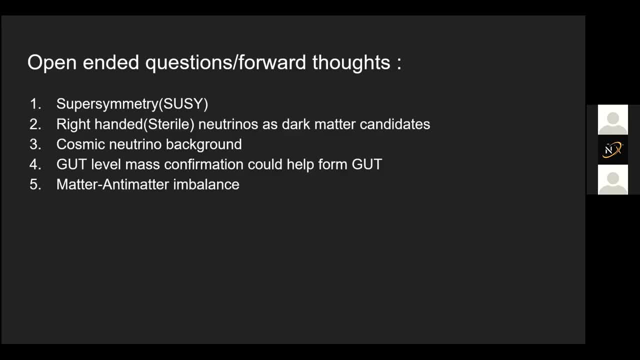 like a super symmetric part of the left-handed one, for example. that could be like a theory, or if you, if, uh, you know, if it's its own antiparticle, like a major, or nothing is right, then the right-handed and the left-handed neutrino are the same neutrino. 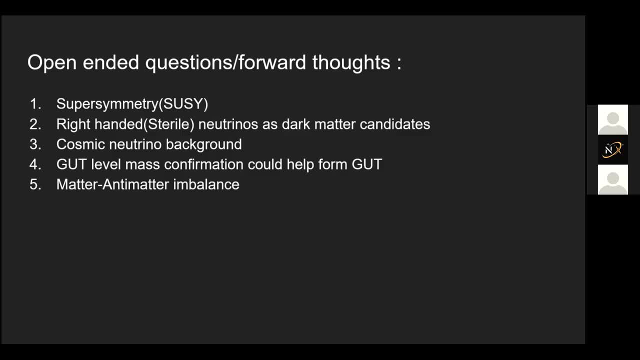 but we just observe the, we just don't observe the supersymmetric brothers of it, uh, counterparts of it. so, like the sterile neutrinos, like the heavier neutrinos, the m, the eigenstate, the positive eigenstate, that m2 uh eigenvalue for the majorana mixing thing, if you guys remember that could be the. 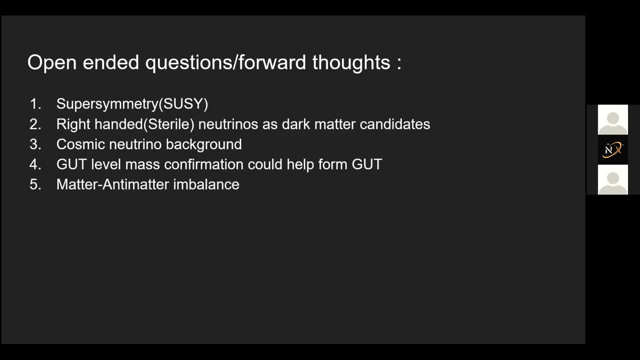 supersymmetric counterpart of the l. so maybe we have found, you know, right-handed neutrinos, but it's, but we just call them anti-nutrinos, but supersymmetric, could you know, prove otherwise? so another one is right-handed sterile neutrinos as candidates for dark matter. 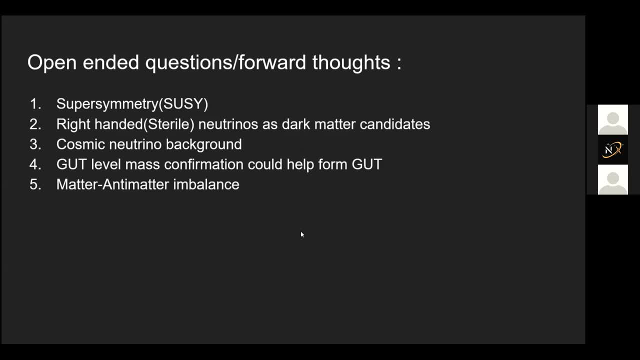 now they're called sterile because they don't interact with anything. and if they do have, you know, higher mass, that the gut level mass, uh, those could very well be candidates for dark matter, because we know that, i mean as of now we know that dark matter does not correspond to the 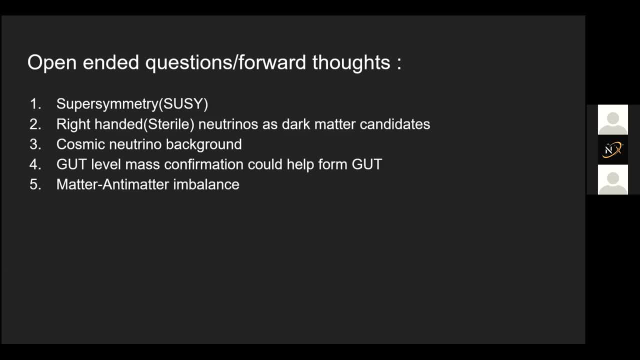 not interact in any means whatsoever except gravitationally. so a sterile neutrino would be a very good you know candidate for it. because it's heavy, it doesn't interact with anything, and because it's heavy it could be dark matter, you never know. and the cosmic neutrino background. 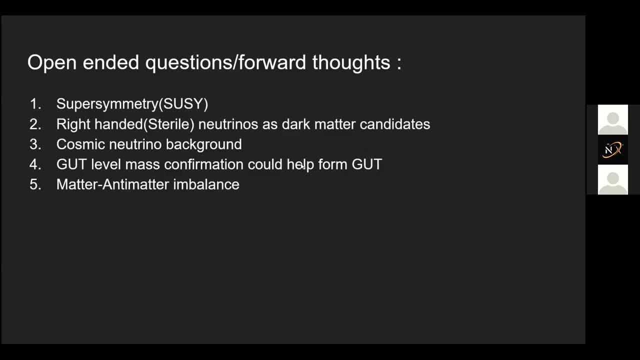 this isn't exactly so much so as any of the standard model failures or possible thoughts. this is just a very uh open-ended or a very theorized thing in the field of neutrino astronomy. uh, it's the fact that, uh, we have the cosmic microwave background right, that we've predicted. 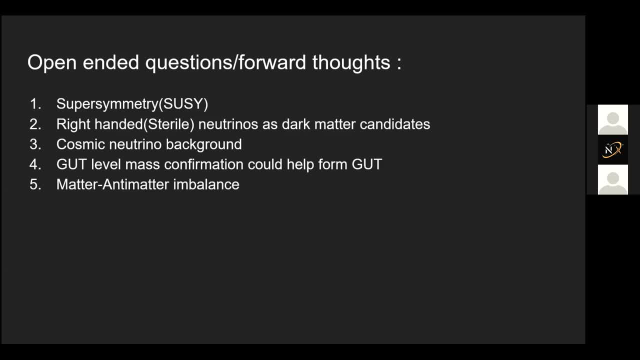 that to be uh, what, uh, about a few hundred thousand years after the universe has been born? the reason why we can't get an earlier image is that the universe was so dense before that that no photons could escape, you know, but uh, neutrinos, they don't interact with matter as much at all, so 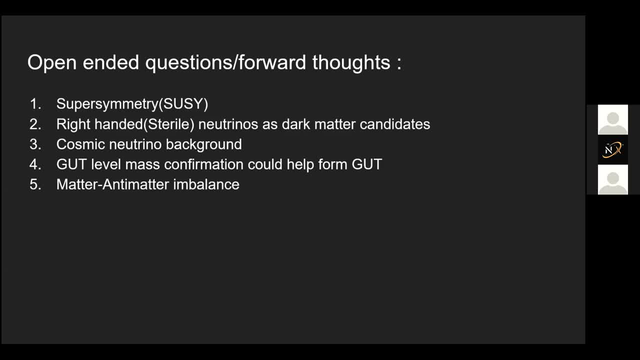 neutrinos could have escaped way before it. so if you do find a way to collect this information, if you do find a way to detect them- you know, currently they say it's near impossible- it's supposed to be 10 to the minus 5 electron volts, something like that it's supposed to be. 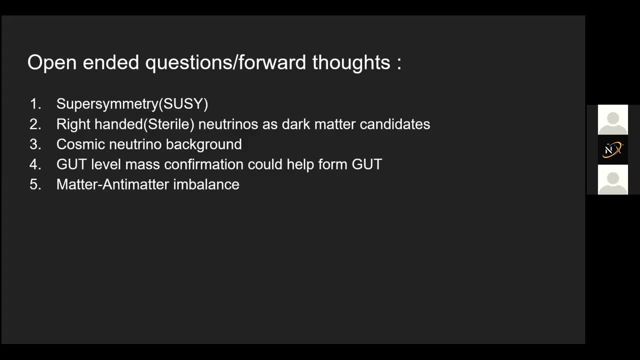 very, very. uh, the high energy ones are supposed to be very low energy, surprisingly so it's very hard to detect, but if we do do it then we could get an image of the universe as young as one second old. that is an amazing thing for the field of astronomy, astrophysics, cosmology. just understanding. 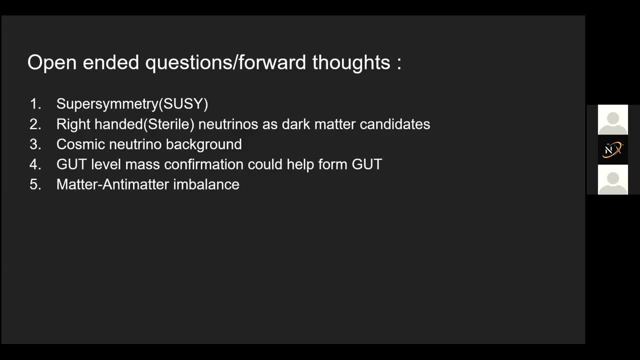 the universe, there could be a great break through. it has been theorized but it has not been detected yet. that's the cosmic duty in the background. the gut level mass confirmation could help, uh, form the gut. if you have gt level, uh, a grand unified theory mass, then if you build physics upon, you know, using that mass as a general case. 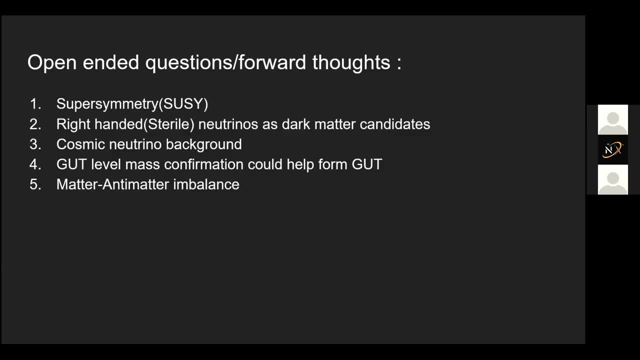 then you could actually form a grand unified theory, because at that scales gravity would indeed dominate and we've already seen that via the weak force and the major runner and mechanism that those heavy particles can exist. so it would be like a way to help inch closer to trying- and you know, mixing- 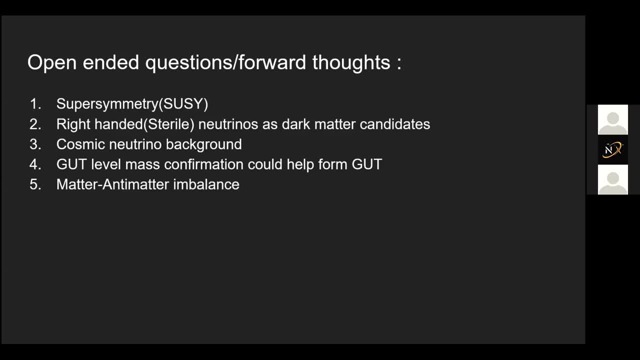 gravity with the quantum mechanics, the one thing that nobody has been able to do ever. that would help, really help form the grand unified theory and hopefully einstein would be happy. and another crazy thing: believe it or not, the charge parity violation could even answer the matter, antimatter. 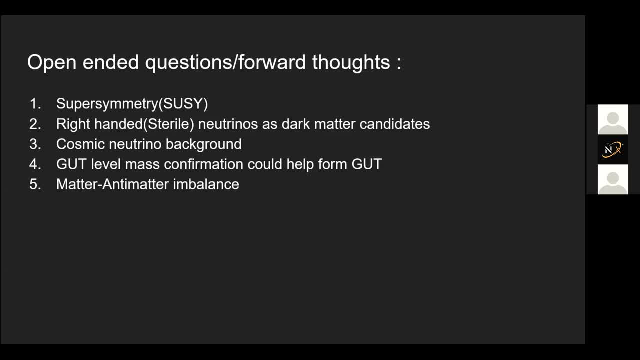 imbalance in the universe, because so far, everything that we know of is, you know, symmetric: there's equal quantities of this and equal qualities of the opposite of that. but the charge parity violation could very well say why. uh, by the right and left are obviously just conventions, but once we stick to it, we have to stay, so a matter which is left-handed would 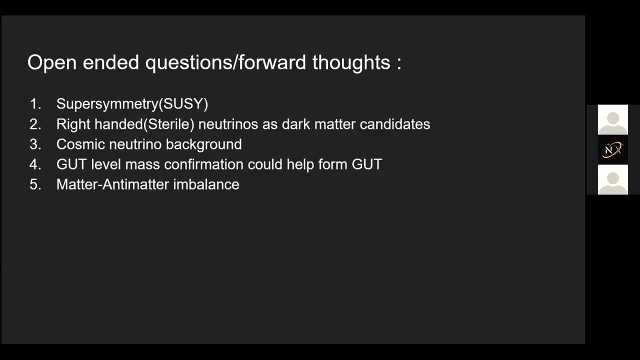 take over uh, more of the universe. because this sort of violation, the tendencies for decays and such, would explain the stability in early universe universe, the neutrinos that we can get from early universe, if we can, can further tell what mechanism was at play when we got this imbalance in the first place. 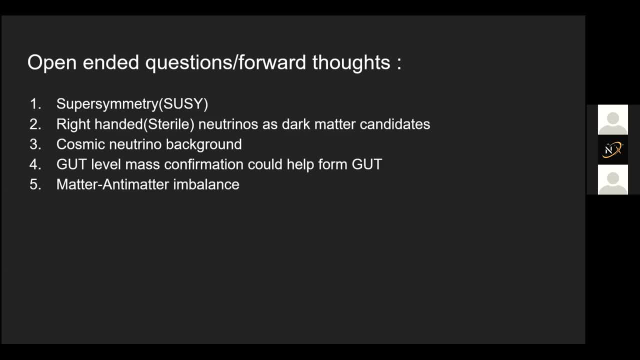 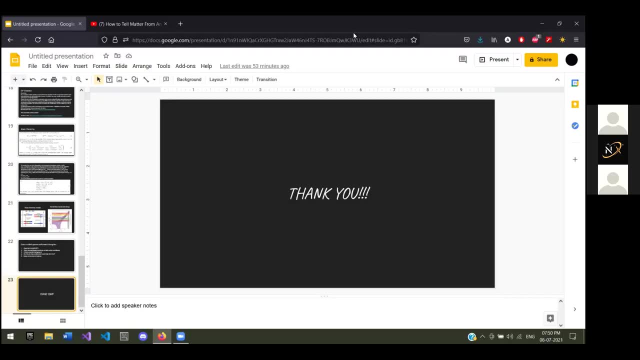 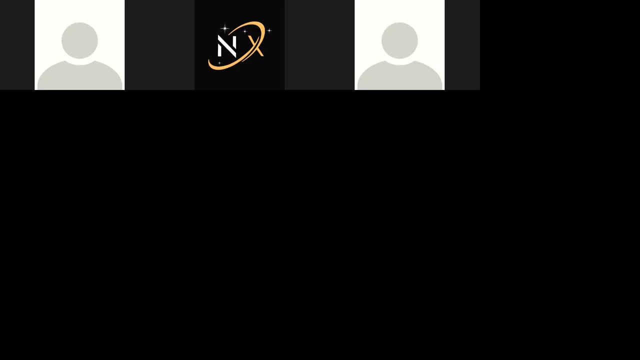 So these are some open-ended questions related to neutrinos, their masses and extension of the standard model, And I hope you had a fun time. Thank you, You can ask questions now if you want. Yeah guys, I'm done. Is there anybody you want me to go over again or any questions? some feedback: 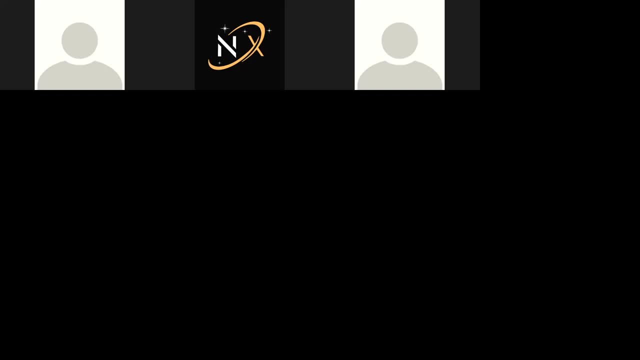 So, Aditya, it was a nice presentation and actually I understood many of the topics which I couldn't understand in Wikipedia. but so thanks for explaining, Aditya, and so does anyone have any questions? Or do you have any questions, Any doubts, or you want to say anything? you can unmute and ask now. 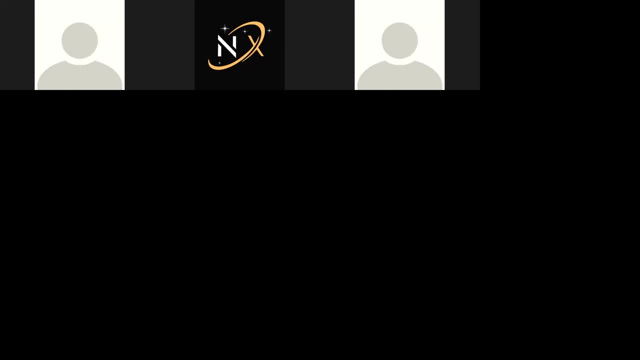 Thank you, Sadgur. And yeah, guys, you can ask. Okay, so I think nobody have any doubts. So how about Group two people? if you're here, you tell who was the presentation. Is there anything to improve on that?